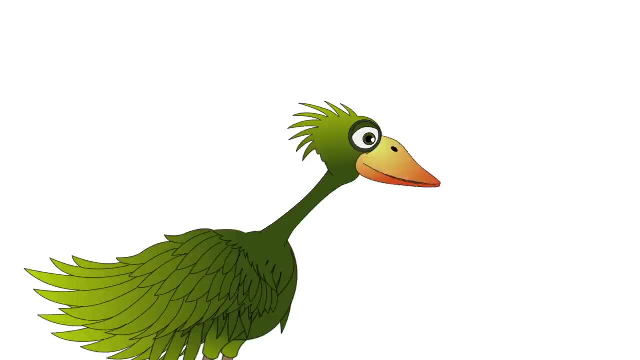 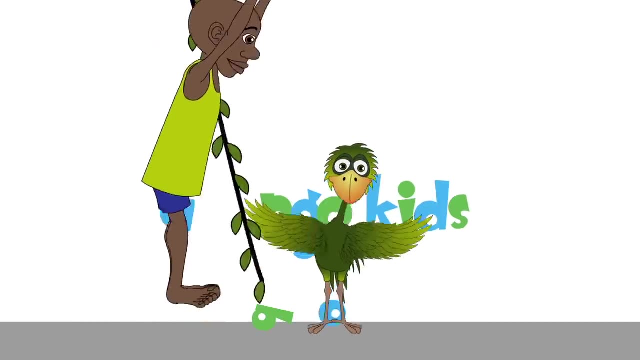 Hey, Who is that trying to To bash down that wall with their head? You know there are other ways to use your head To solve a problem. That's true, Mom and Deggie. They can try different ways and practice. 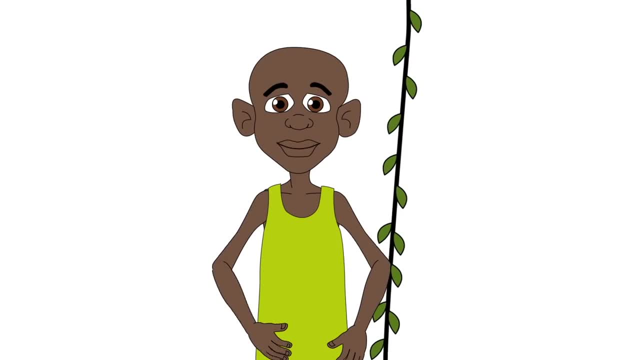 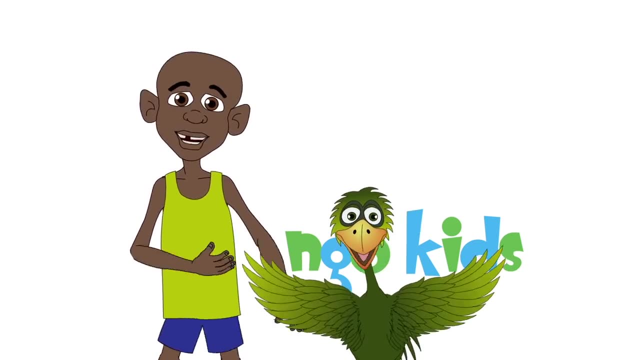 Your brain can learn and grow. It's called having a growth mindset. Grow your brain, grow your brain, give it work to do. Grow your brain, grow your brain, learn something new. Grow your brain, grow your brain to be a smarter you. 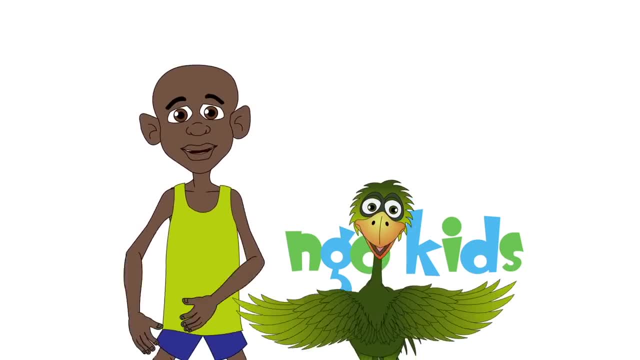 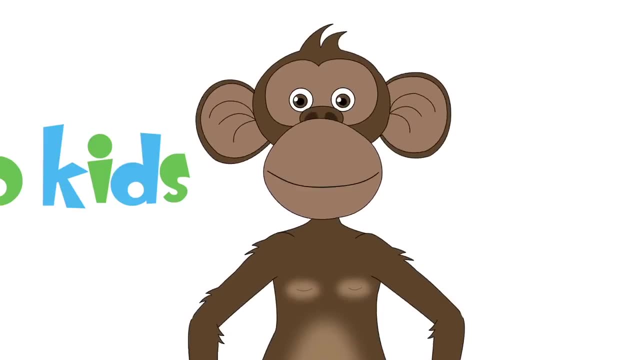 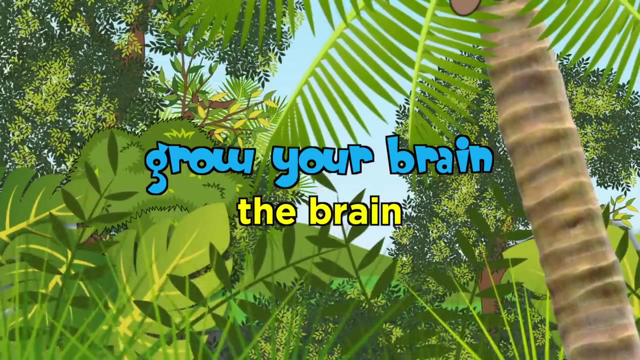 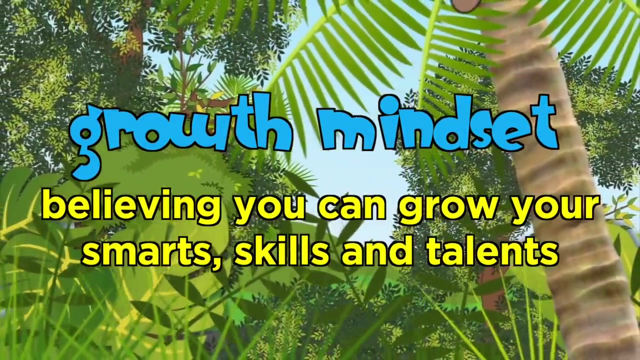 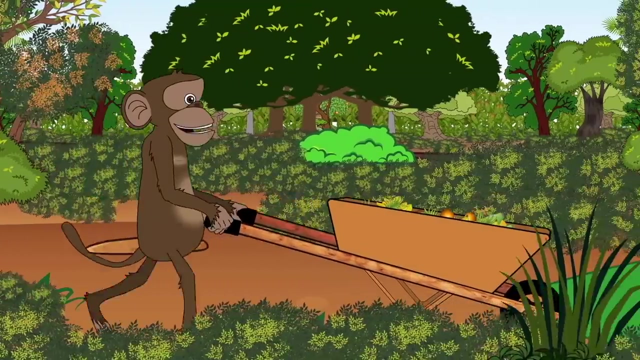 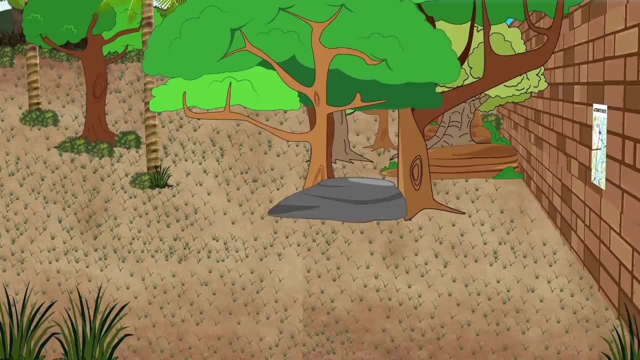 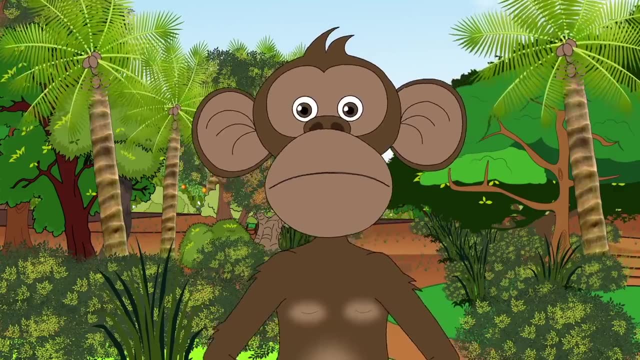 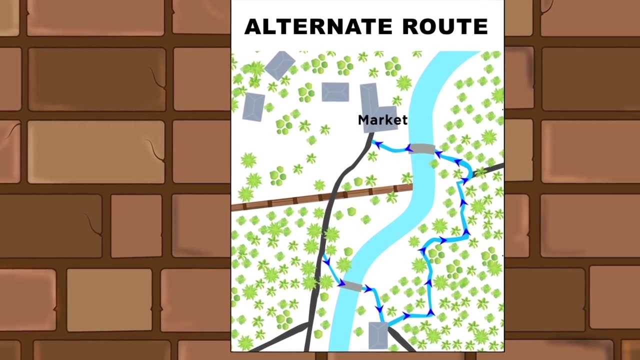 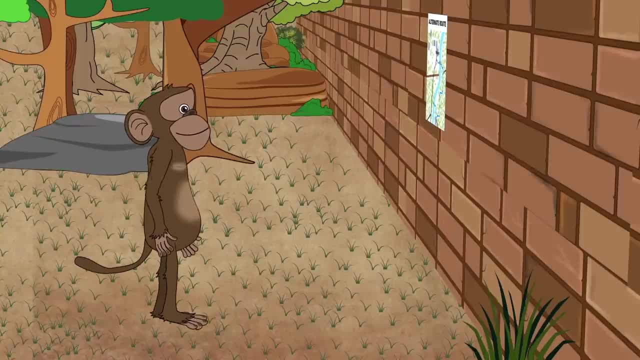 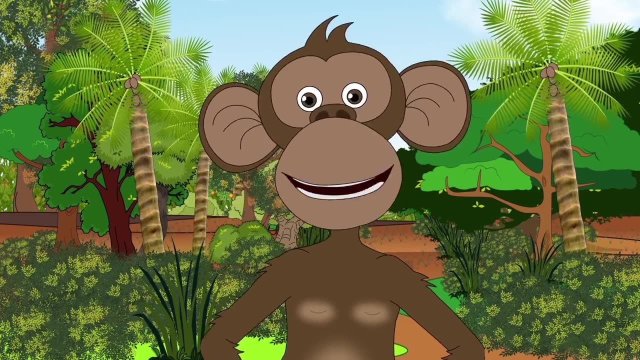 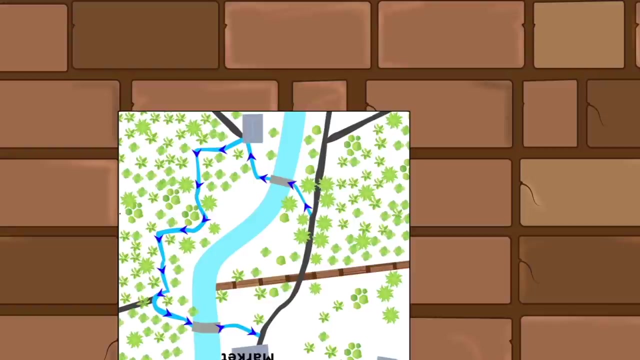 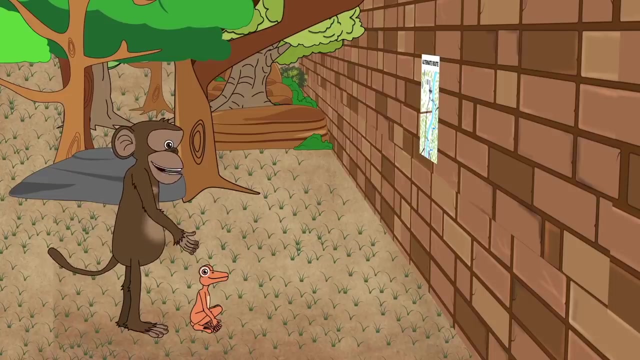 Huh, Huh, Huh, Huh Huh. Alternate route, alternate route. Hmm, let's see. Oh no, can I hear it Da Jura Hi. So are you going to take the alternate route? 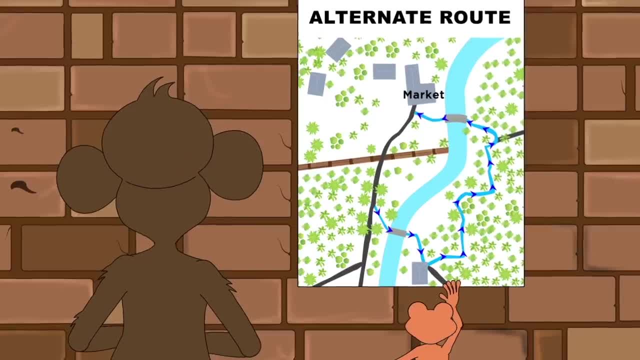 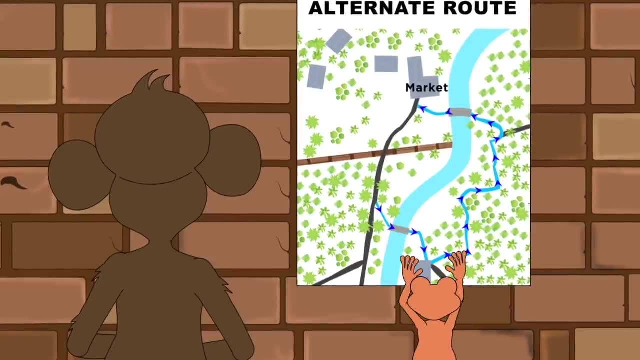 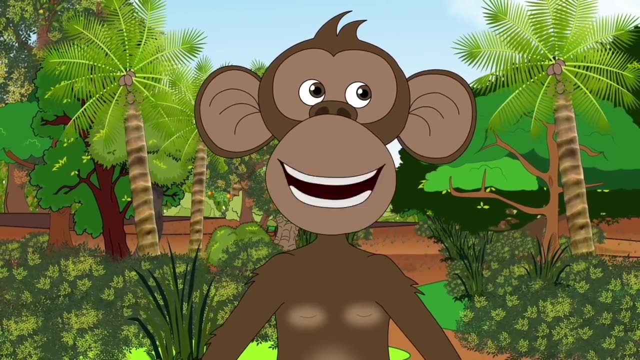 The trail, Cross the stream, Turn right and through the coconut trees, Left, left, right, left, over the hill and down the road. Looks easy enough. Oh yeah, looks like a piece of cake, So you're going to go. 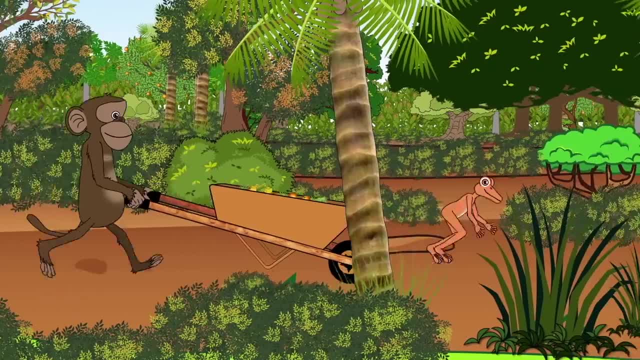 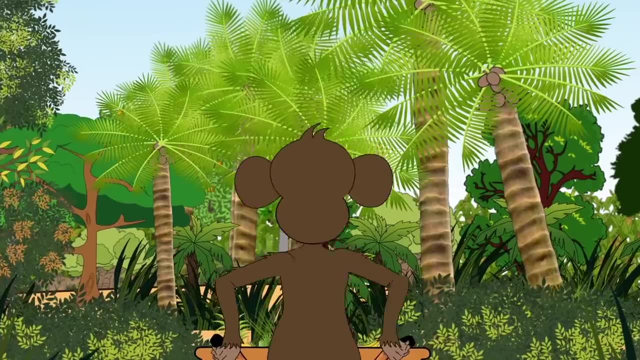 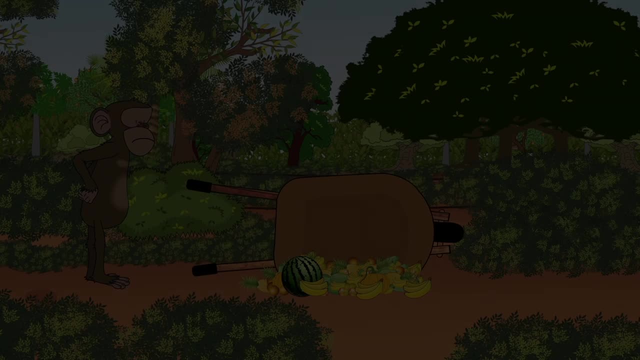 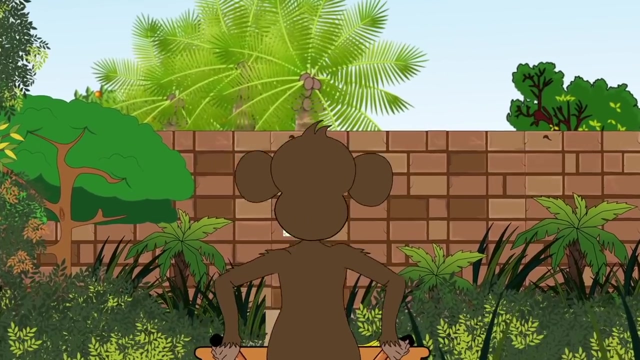 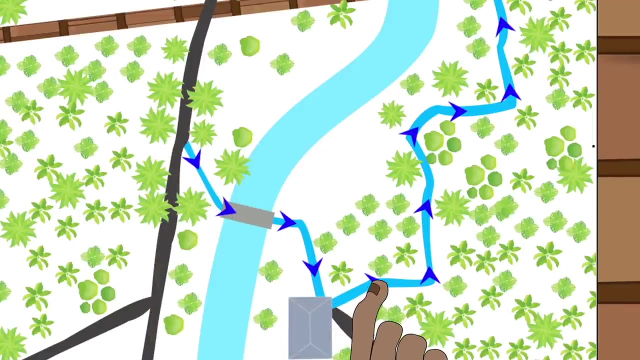 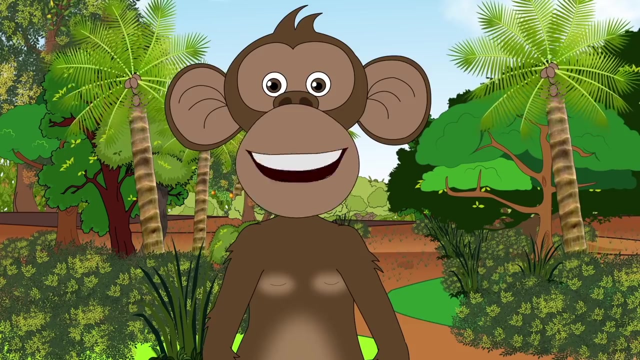 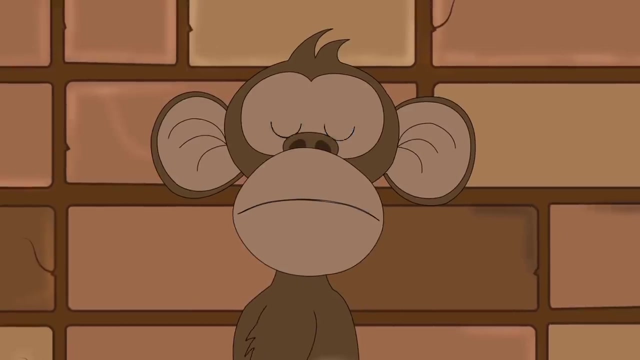 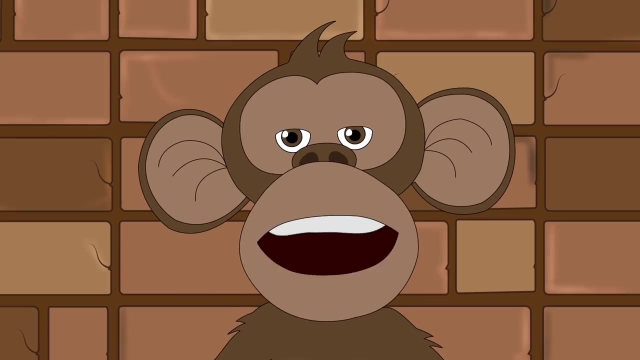 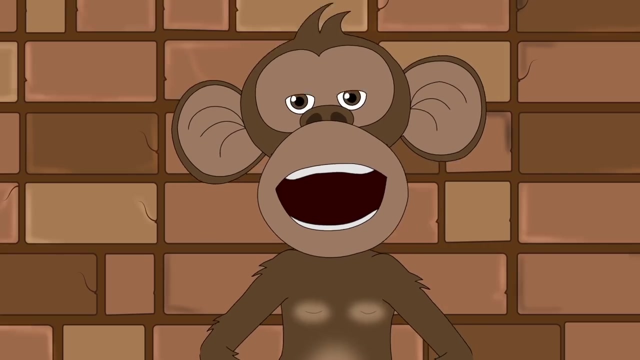 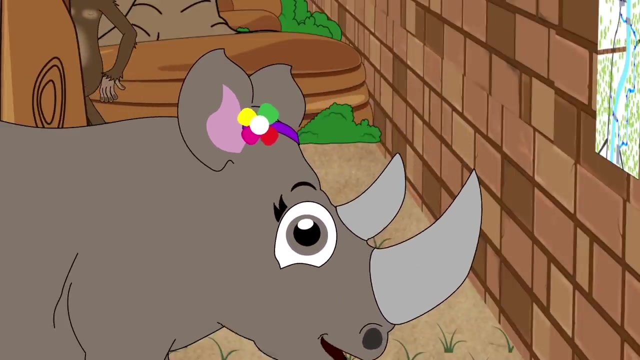 Sure am. Hmm, is that a dachura Mamandege? I can't read the map. I guess my brain isn't big or smart enough. Uh Huh, Aw, it's still standing. Oh, better try again. 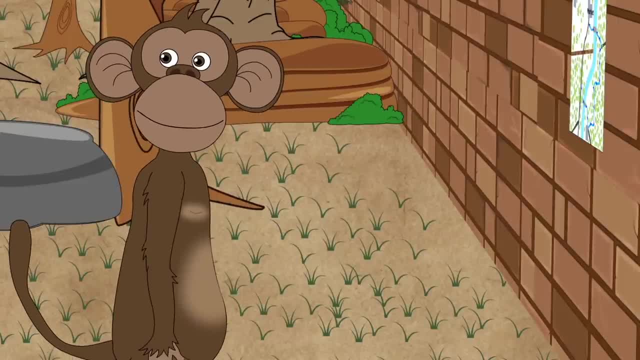 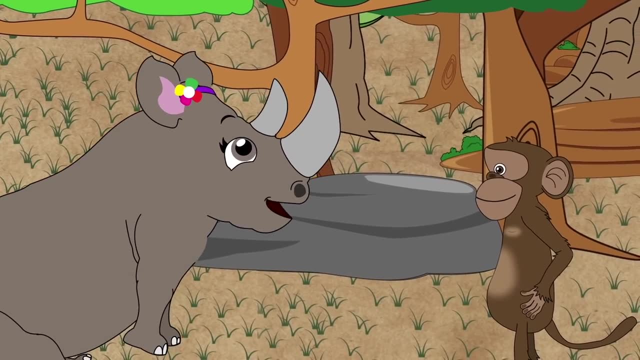 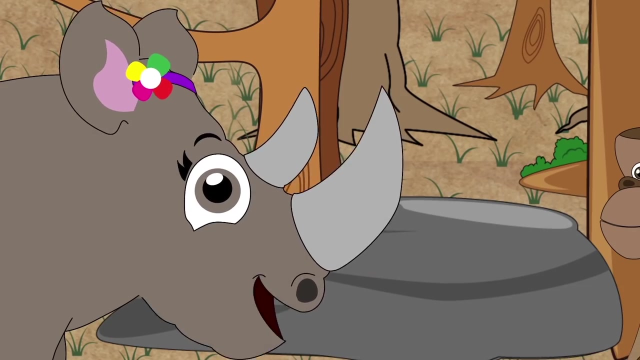 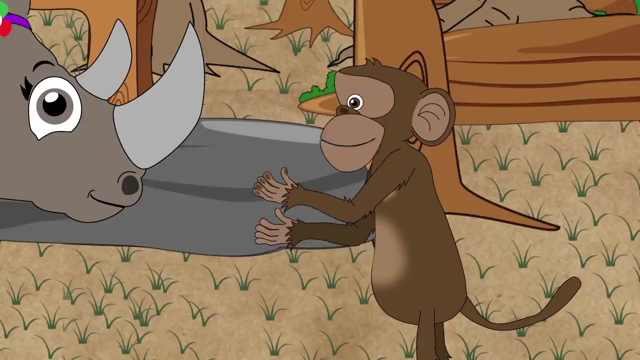 Out of the way, Are you alright? Yeah, I'll be okay, Just gotta shake it off. Who are you? I am Gedere. I sell fruits in the market and use my profits to buy- guess what- pilaf. But I can't get there now because this wall is blocking the way. 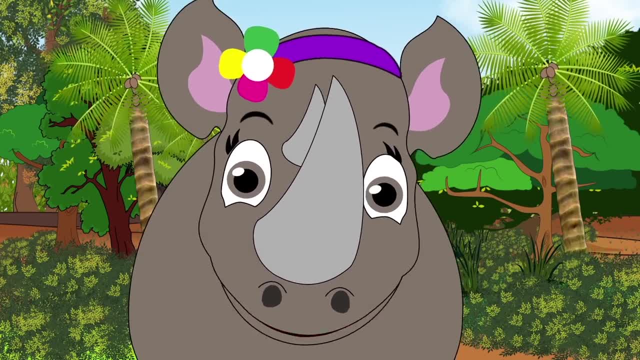 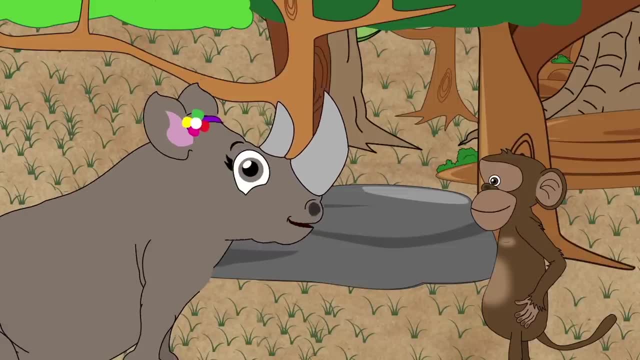 Nice to meet you, Gedere, I'm Faradia Faru, but people call me Fafa for short. I'm trying to get home, but this silly wall is in the way, So I'm gonna knock it down. I don't know, That's a pretty big wall. 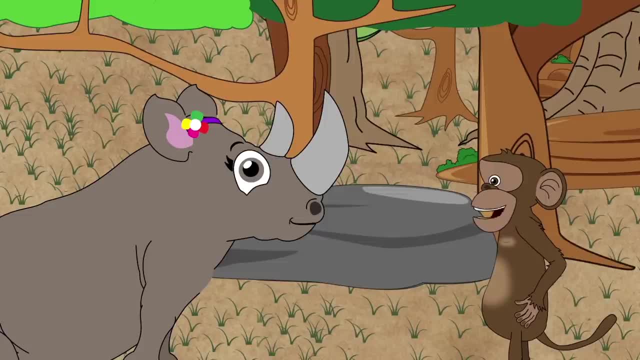 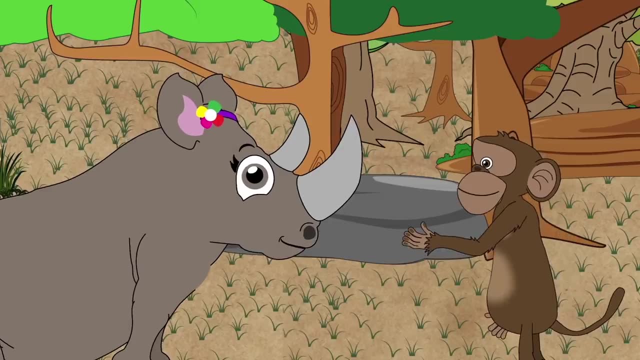 If we can read the map, it shows us another way. My brain isn't big or smart enough to understand all that, But look at you. Your head is huge. You must have a really big brain. I bet you can read the map. 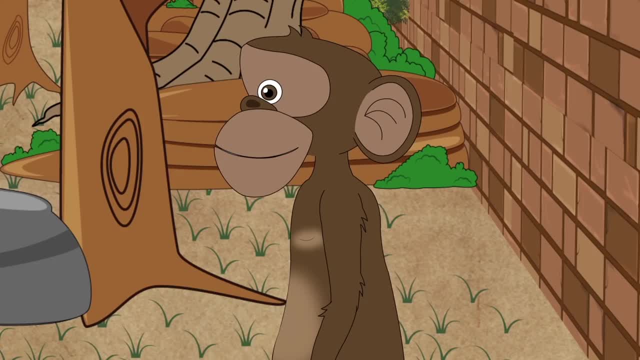 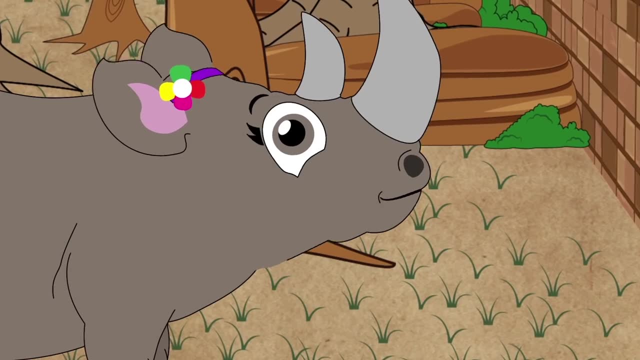 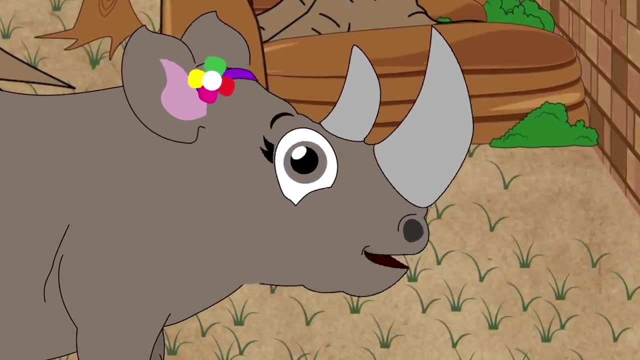 Nope, No idea what any of that means. I'm good at bashing- Really good at it. My daddy says I'm the best young basher in the whole forest, So I'm gonna bash this wall down. Maybe I can help. 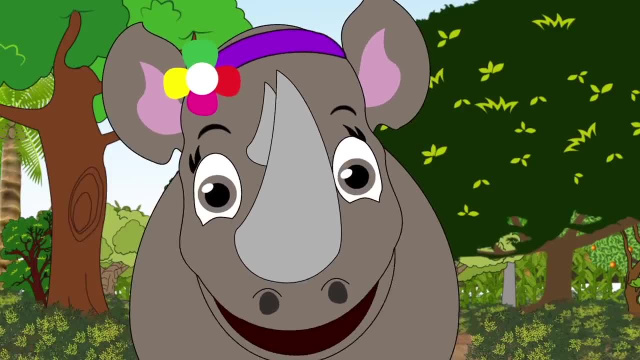 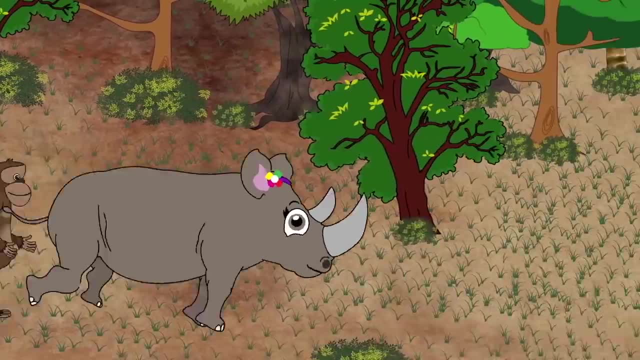 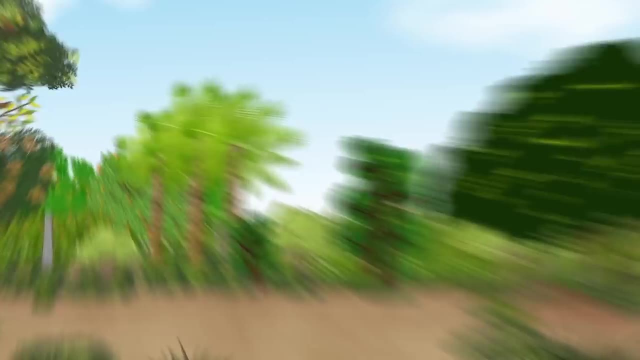 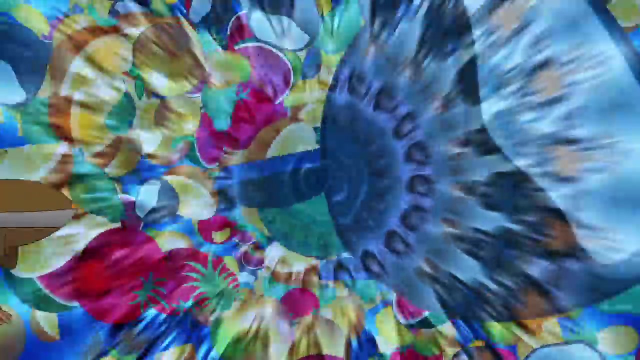 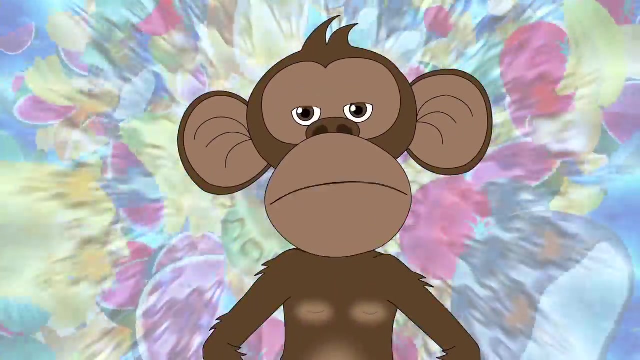 With that little head. Well, you could try. I guess I am your brain. You think the brains won't be able. We can grow until we've got to help them. Huh, Where am I? We're in your head. 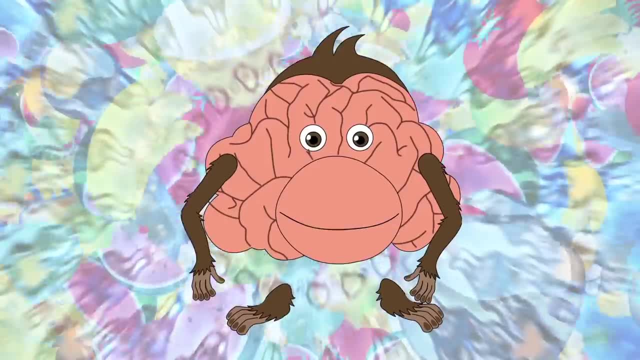 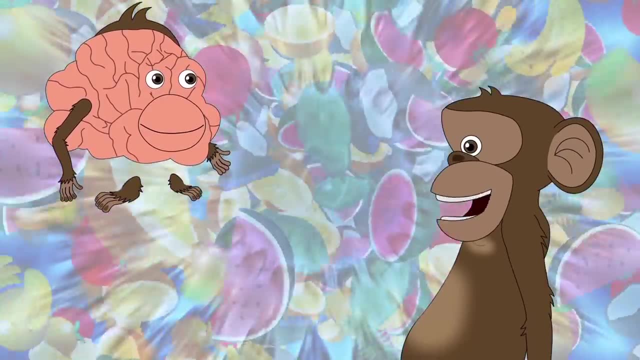 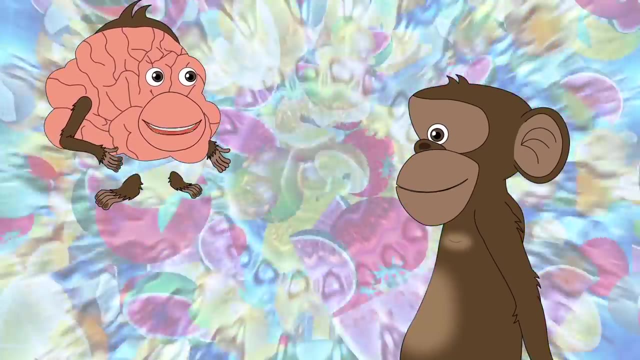 In my head. And who are you? I am your brain. You're the reason I can't read the map. You're too small and stupid. If you are big and smart, we could read the map. Hmm, The only reason I'm small. 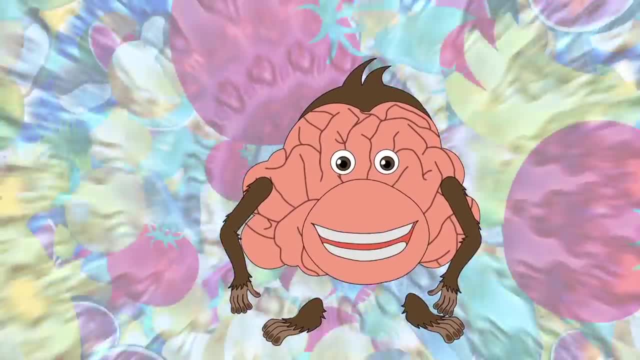 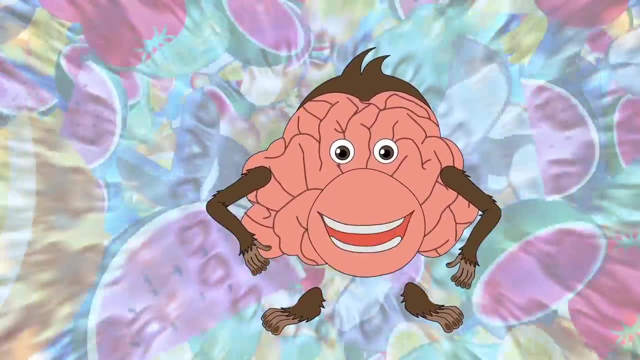 Or, as you say, stupid Is that you haven't trained me or fed me or given me exercise. You think brains grow on their own. Well, they don't. We brains are like muscles: We can grow, but you've got to help us grow. 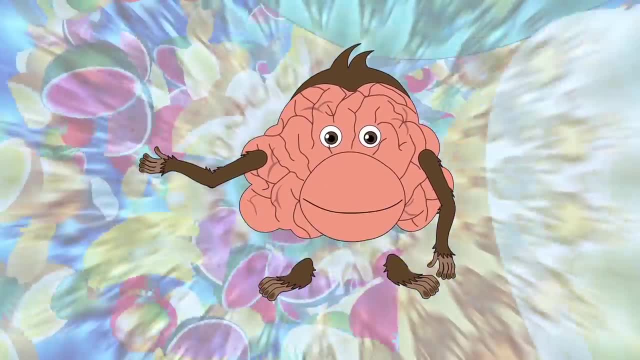 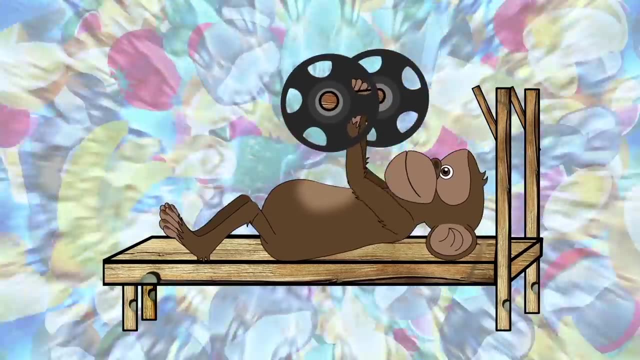 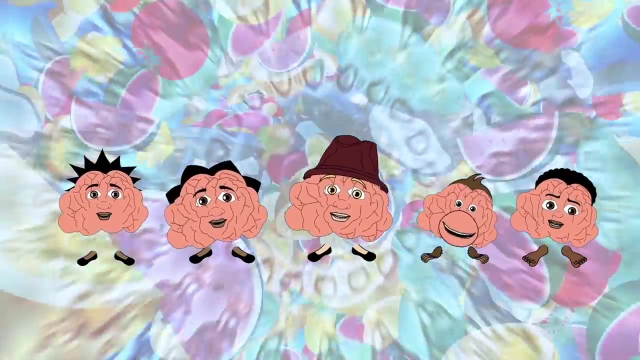 Hey, little monkey, did you know The brain is like a muscle, It can grow. It just needs a little love and exercise So it can grow up to a genius size. Grow your brain, grow your brain, give it work to do. 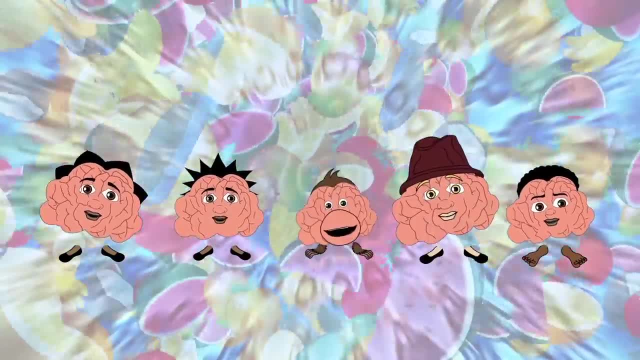 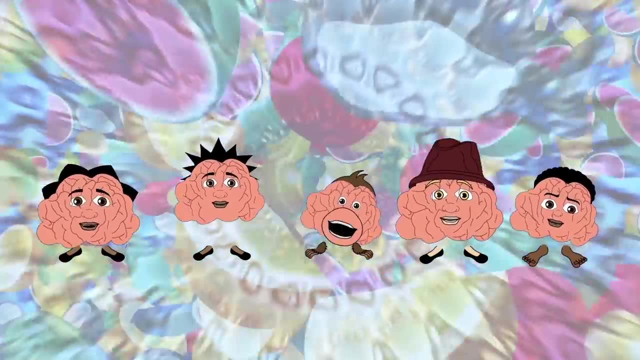 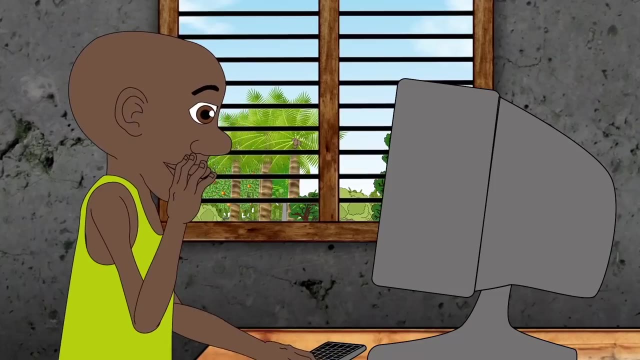 Grow your brain, grow your brain, learn something new. Grow your brain, grow your brain, be a smarter. you Give the challenge a go and help your brain grow. It's true, the brain can grow. it just needs exercise To learn a prime new skill. it takes a few tries. 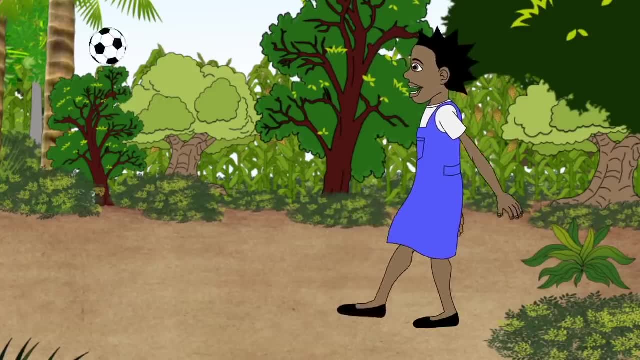 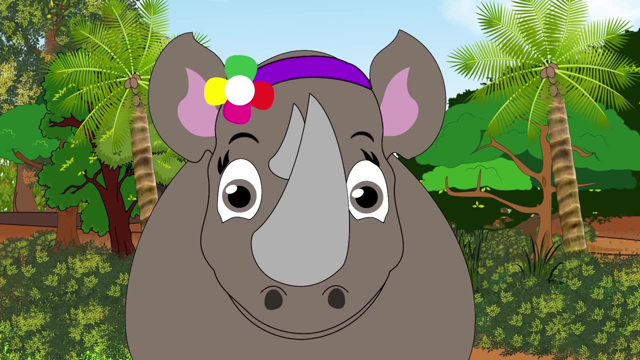 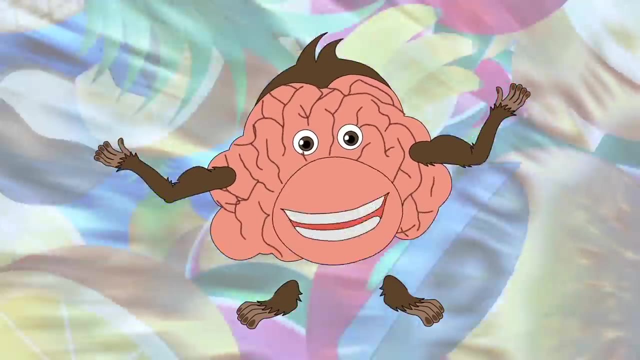 It's not about talent or being born that way. If you try and try again each and every day, Try something challenging, try again and again, Try something challenging. don't give up, my friend. A challenge is the perfect food to make your brain grow. 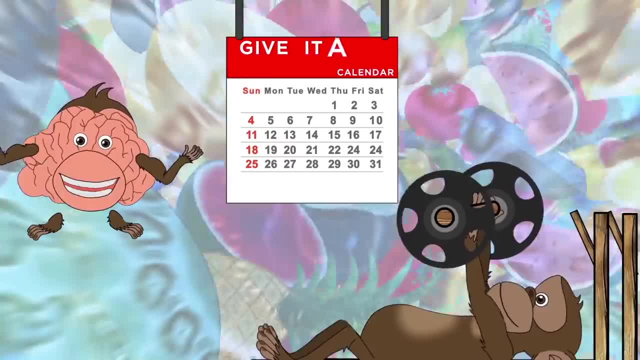 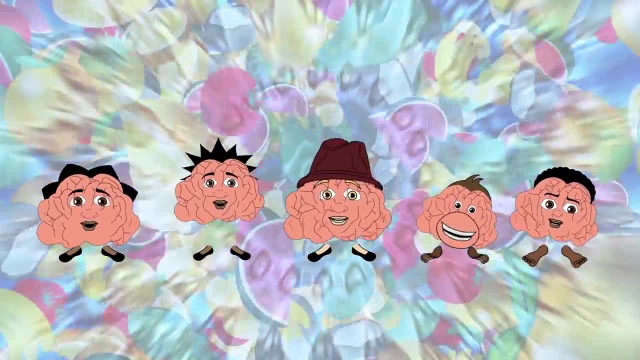 So, each and every day, give it a go. Grow your brain, Grow your brain, grow your brain, give it work to do. Grow your brain, grow your brain, learn something new. Grow your brain, grow your brain, be a smarter you. 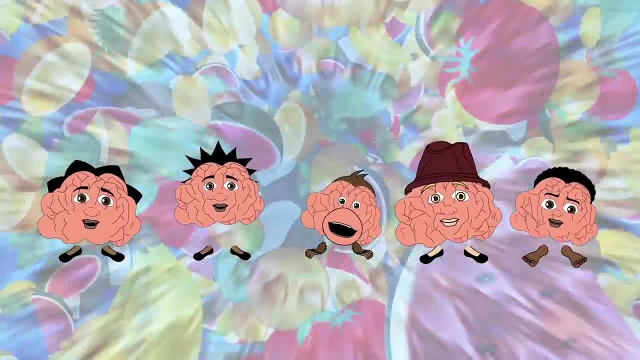 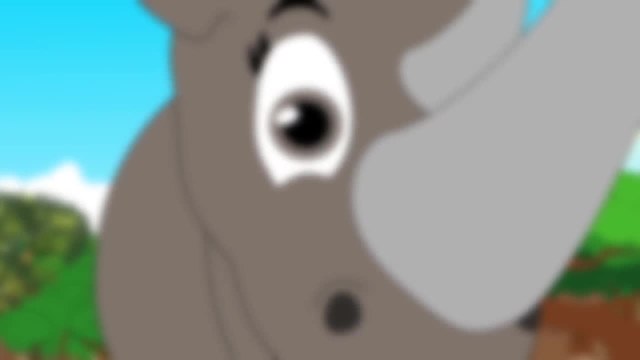 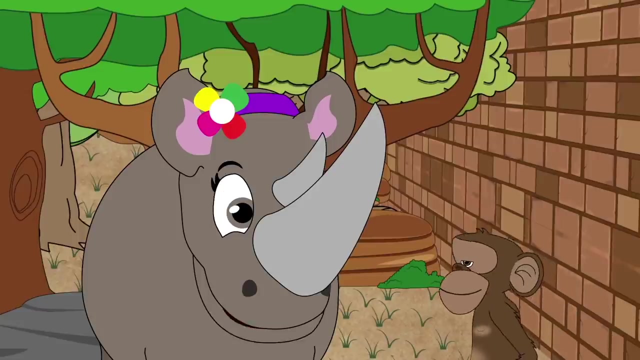 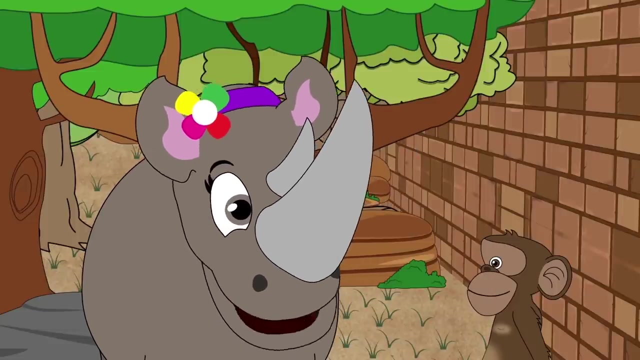 Give the challenge a go and help your brain grow. Gadare, Gadare, Gadare, wake up, Gadare, are you okay? I guess you just weren't born to be a basher like me. You know, my daddy says I'm the best young basher in the whole forest. 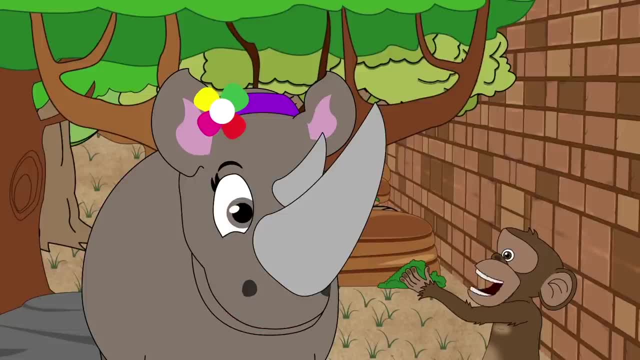 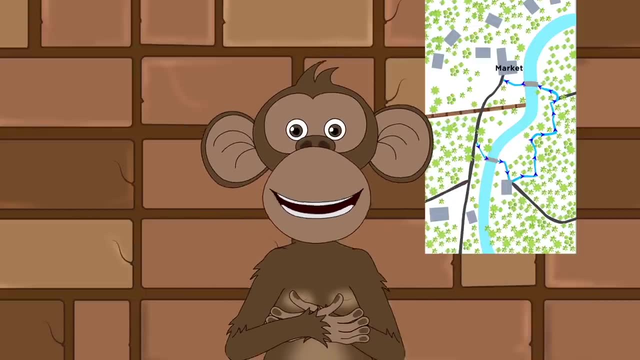 It's what I was born to do. It's not about what you're born with, Fafa. It's about how you learn and grow So we can grow our brains to be smarter, So we can read the map. Come on, let's get to work. 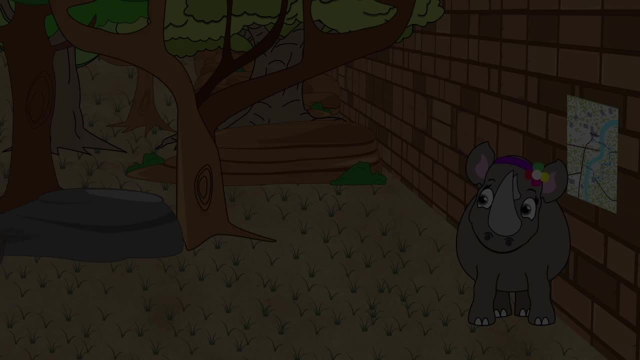 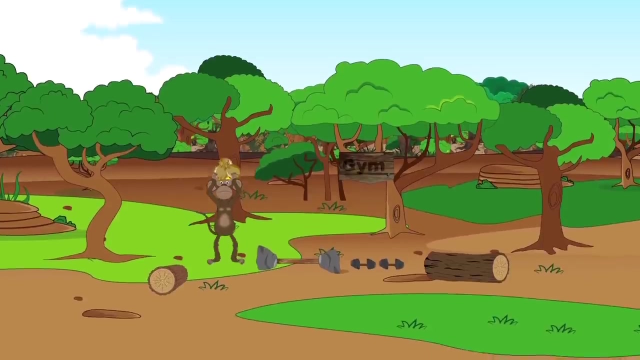 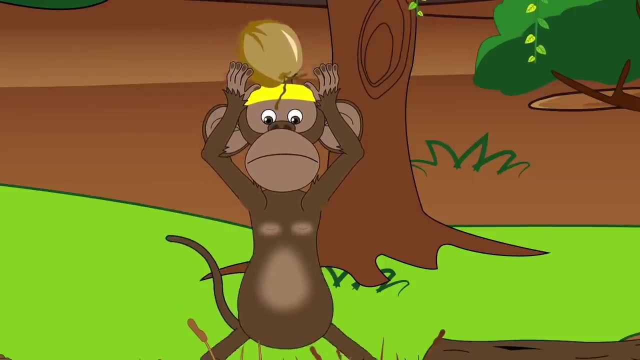 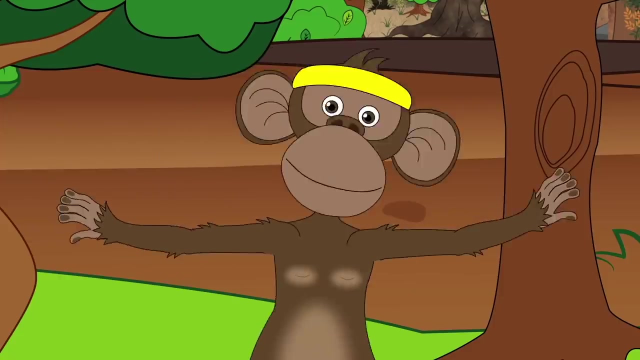 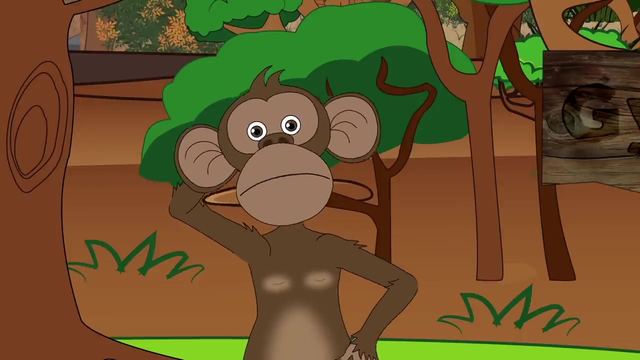 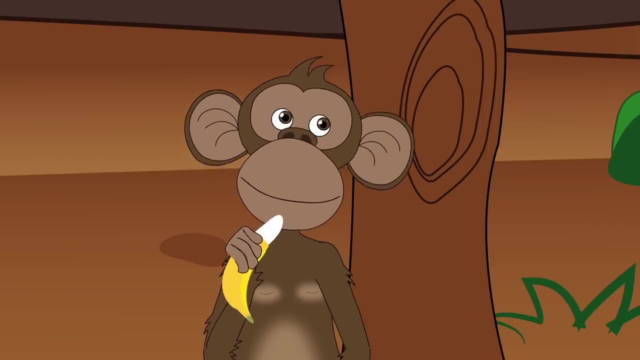 You go, I'm gonna stick to bashing. Hey, brain, um, is this working? I'm not really sure what exercises work for you. So, brain, you're like me. huh, Bananas ain't good enough, You want the good stuff. 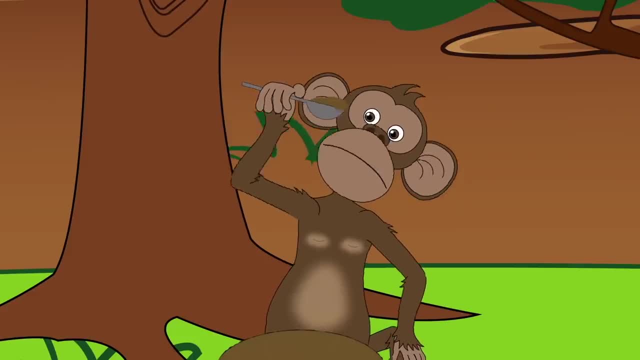 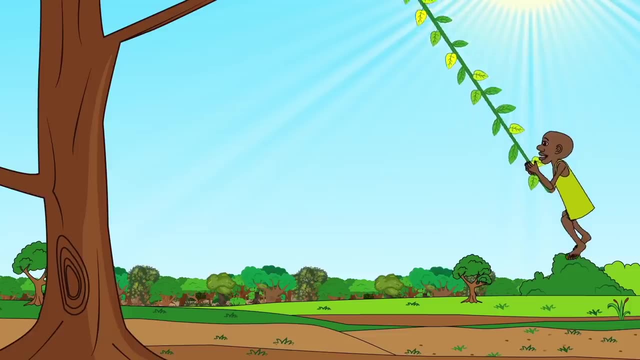 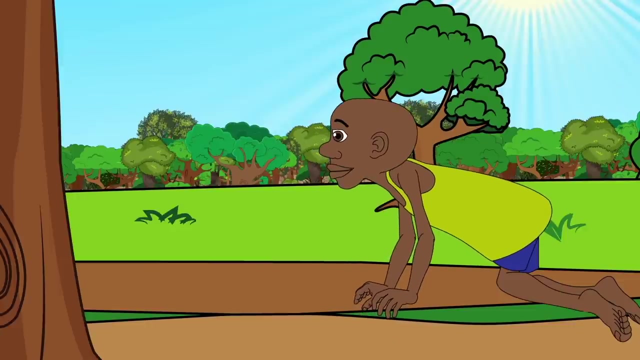 That's right, Man, I don't know how to grow my brain. Wahoo, Ah, ah, ah, ah, ah, ah, Wahoo, Failure number one done. Yes, Hey, Baraka, Um, Why are you celebrating? 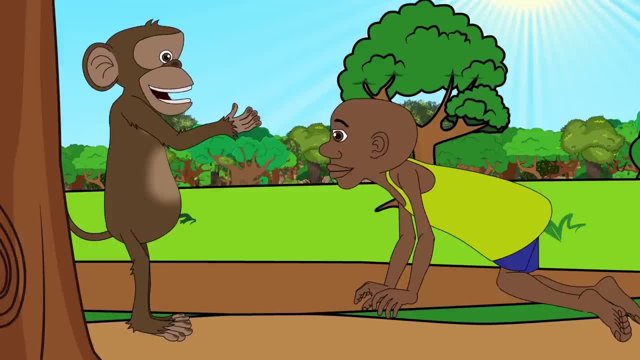 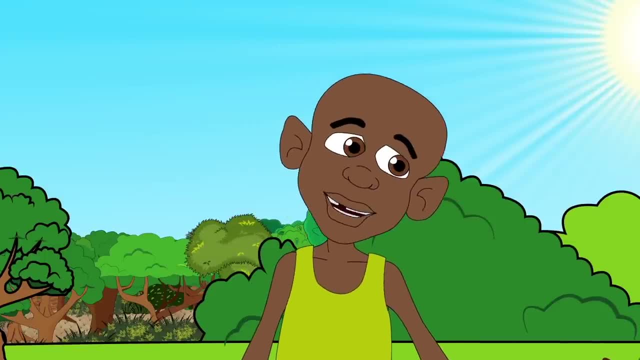 You fell off the vine. Um, you kind of failed. And what is failure Bad? Nope, It's the first step to learning something hard and new. It's how you grow, and it's also fun. Huh, Look at my muscles. 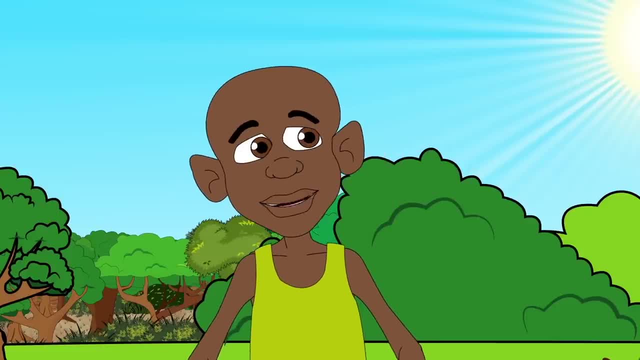 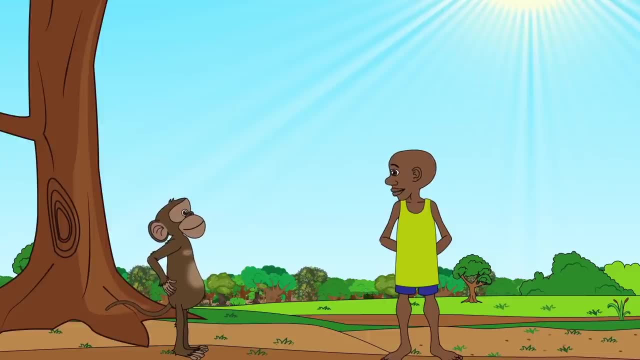 They're small now and I can't swing on the vines yet, But my failure has just shown me that I have something new to learn And if I practice and try the thing, I fail that again And exercise and grow. That's how I learn to do new things and develop new skills. 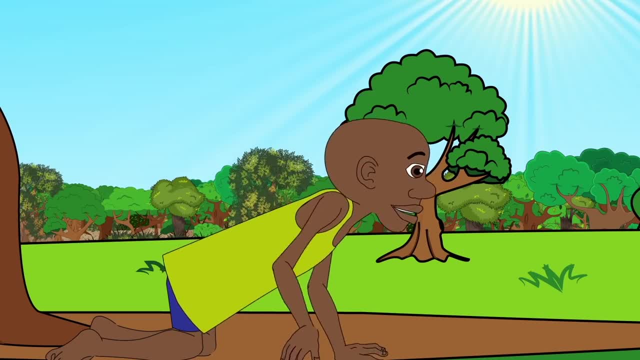 Ow. Failure number two. Wahoo, I'm on my way to be a vine swinging pro, And I can just feel my muscles grow. Why don't you just try the shorter vines, Then you won't fall Too easy? Ta-da. 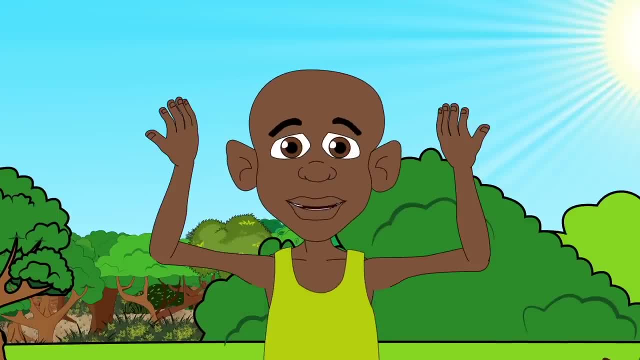 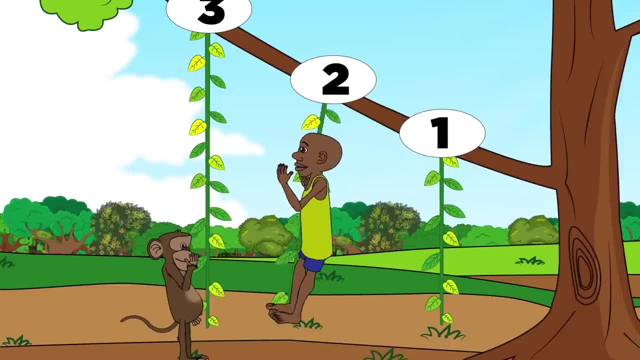 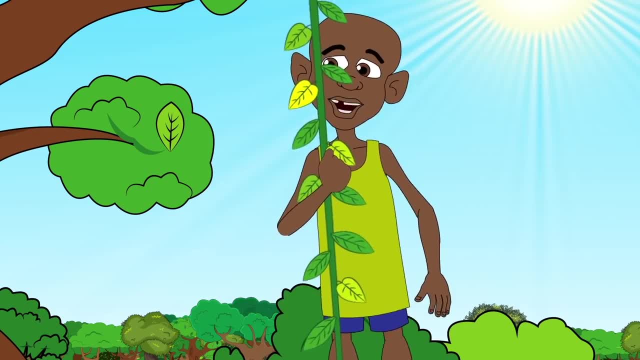 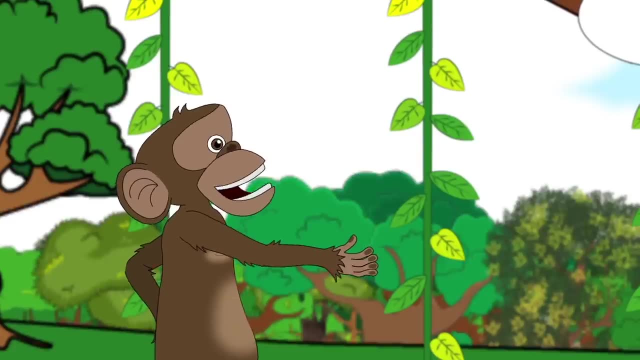 I'm a great viner, Ta-da. If I just kept doing the easy vine that I can already swing on, then I'm not going to get any better, am I? Hmm, So why don't you just go for level ten? 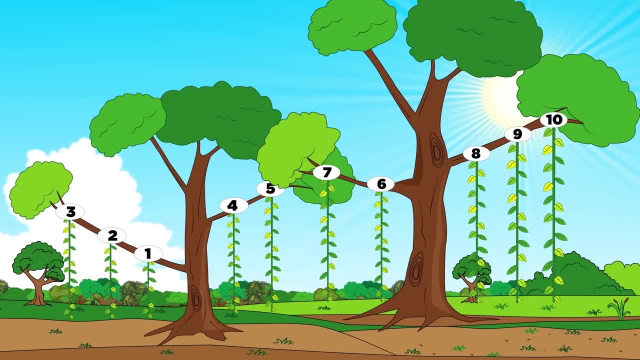 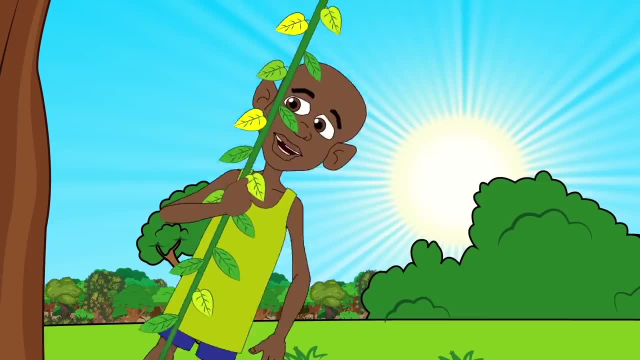 So then you'll get a whole lot better, won't you? I can do level two, but level ten is a big jump. I'll get there eventually, but one step at a time, And my next step is level three. Yes, 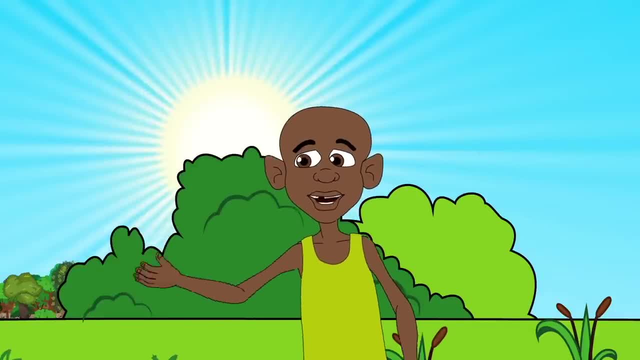 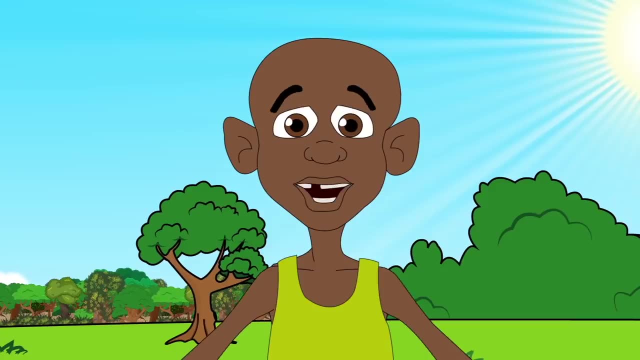 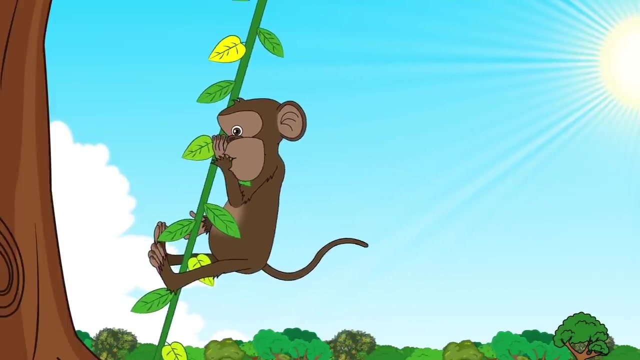 Level three. See how my failures paid off and get everything I want I do. You're on your way to level ten. Wow, Well, I guess I don't need that much practice on the vines. You know, Baraka, I'm actually here because I'm trying to grow my brain. 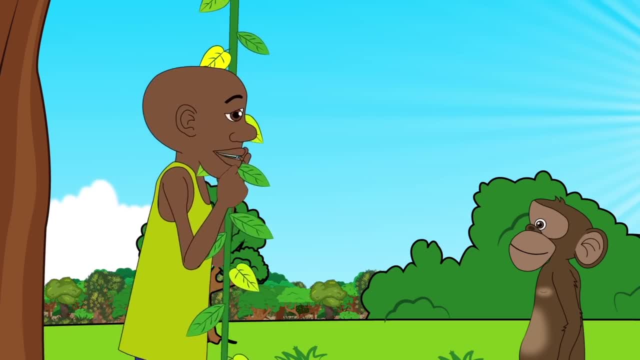 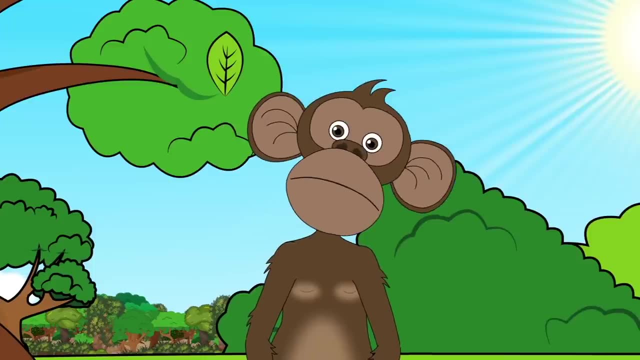 Good for you, Ngedere. I've been growing my brain too. The way you grow your brain is by using your brain to do hard things that you can't do yet. Hmm, But I need to grow my brain first so I can do hard things like reading the map. 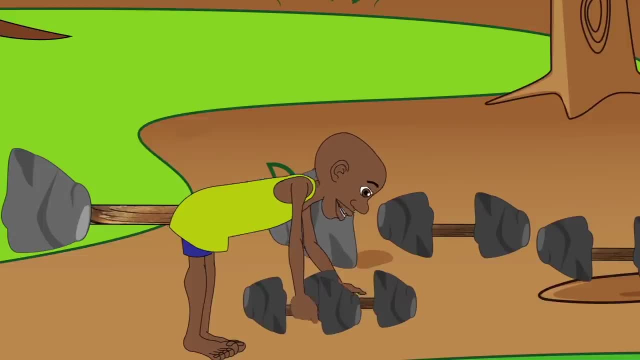 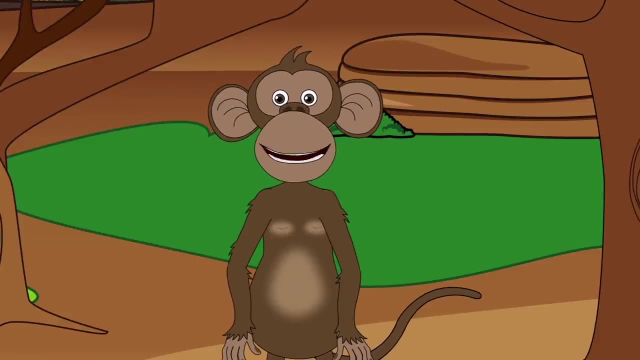 The only way to grow your map reading smarts is by map reading. Ngedere, You've just got to try, But it's too hard. I don't even know where to start. It's okay to start small. You see, I'm starting with the little weights. 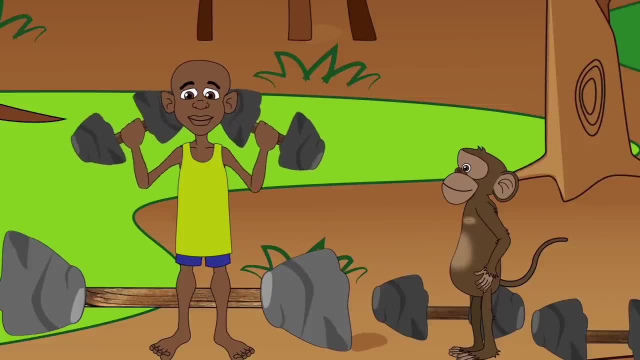 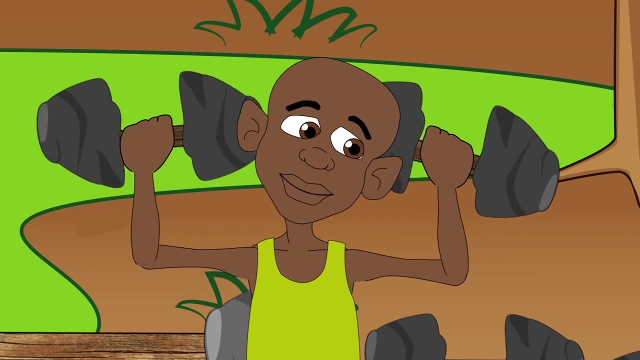 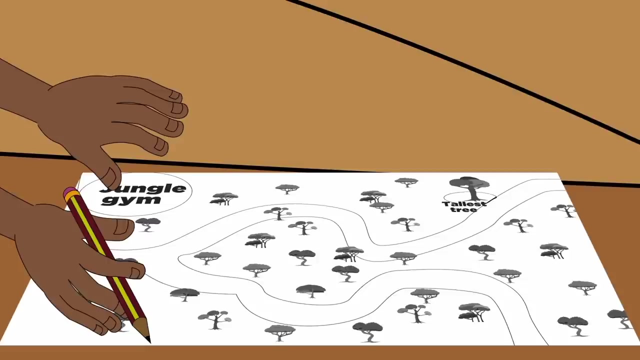 Then I'll work my way up to the bigger ones. So I need a little map, Yeah, And an easier one, Ngedere, I can draw you an easy map to practice with Ready. I don't know What if I get lost. 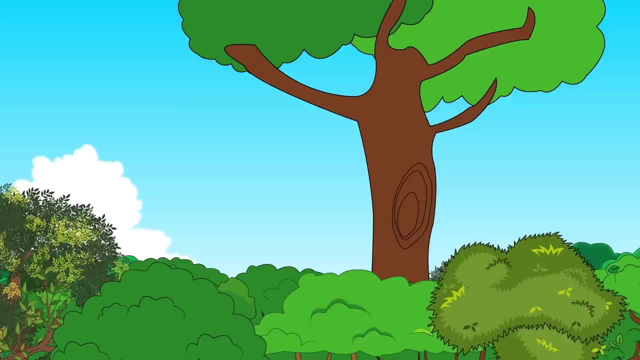 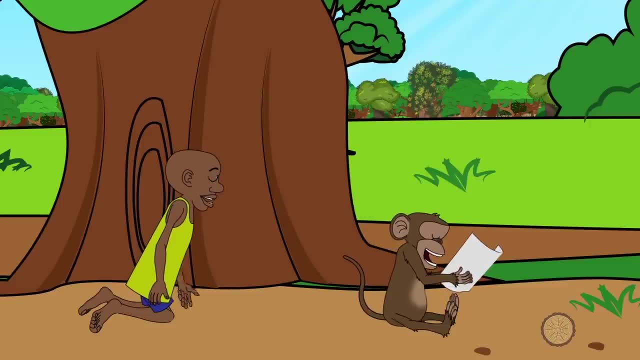 Just look up and look for the tallest tree. You can do it, Ngedere. Don't forget to look up to see where you're going. Yeah, Yeah, Yeah, Haha, Haha, Hahahaha, Hahaha. 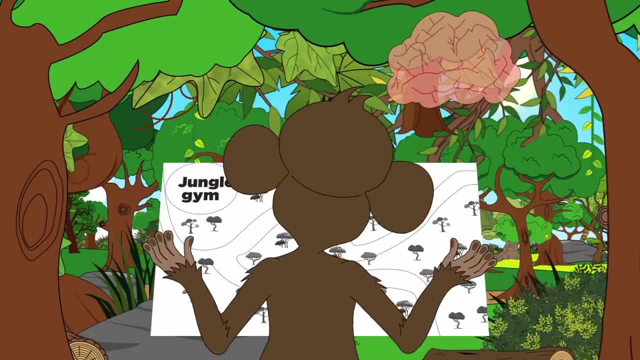 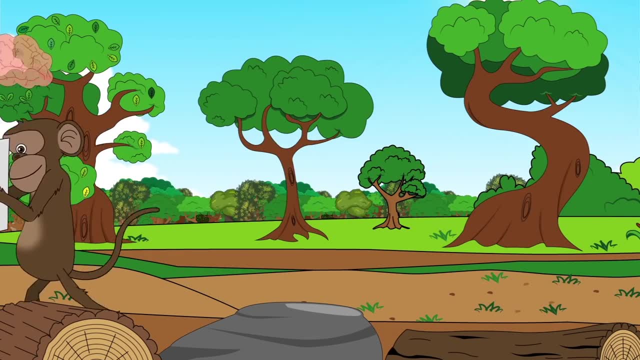 Hahaha, Hahahahaha, Hahahahaha, Hahahahaha, Propertieeees Here And… One, fiftitty And Four, sixty, Let's go Combine, combine, combine, combine. Available at ny Nikecouk. 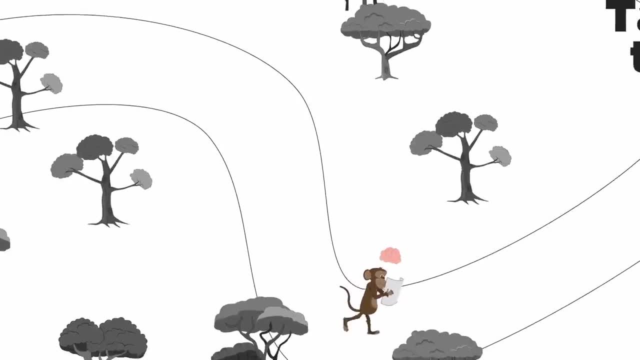 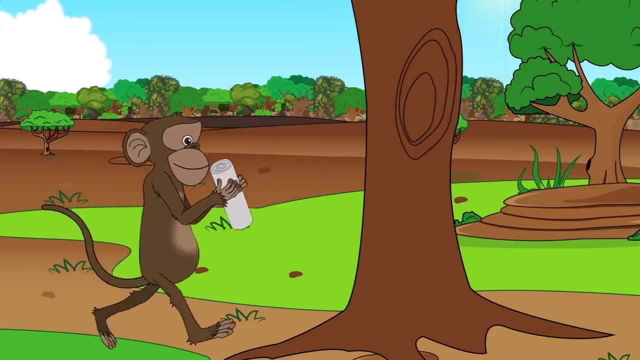 Outboard nail polish. Mm-hmm. anesthetics. Hair hair retirer. Hairstyle maker. hair hair conditioner. hair conditioner. Outdoor nail polish. Hair care bar, Hair remover- Hair remover. My ears are all nice and smooth. 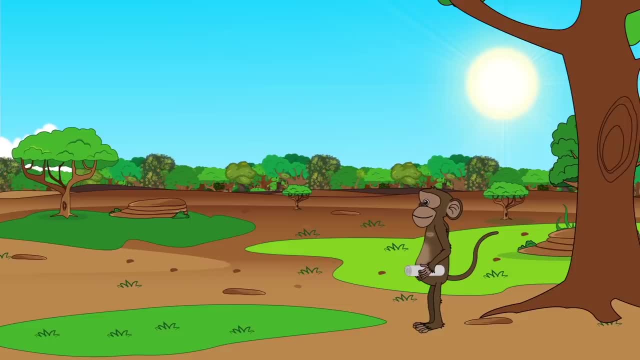 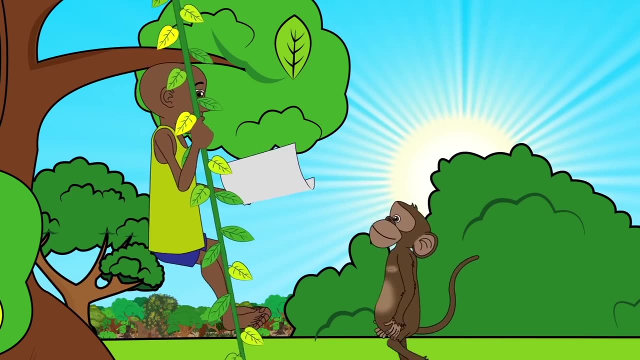 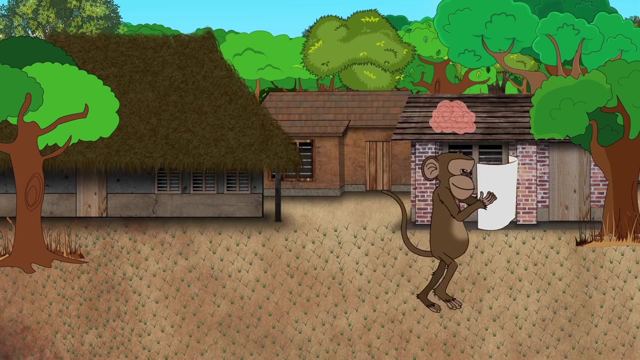 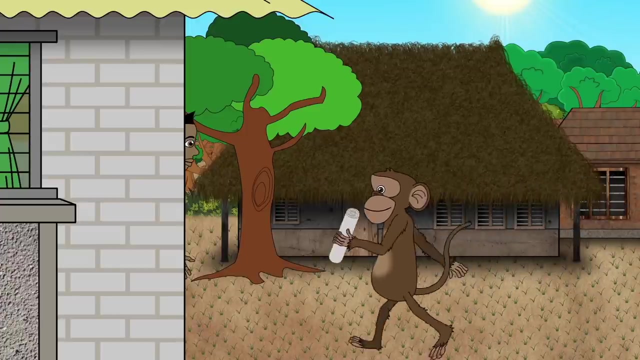 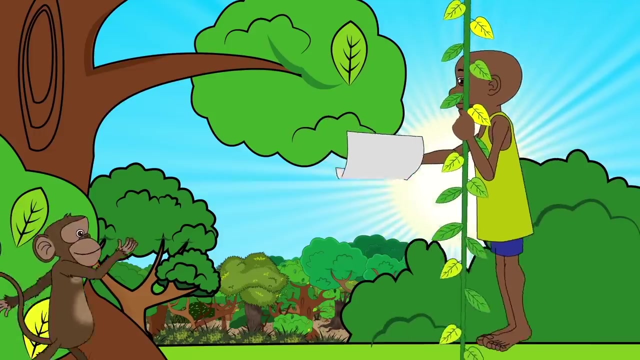 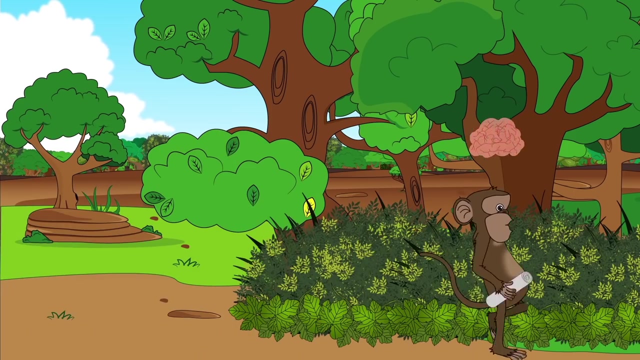 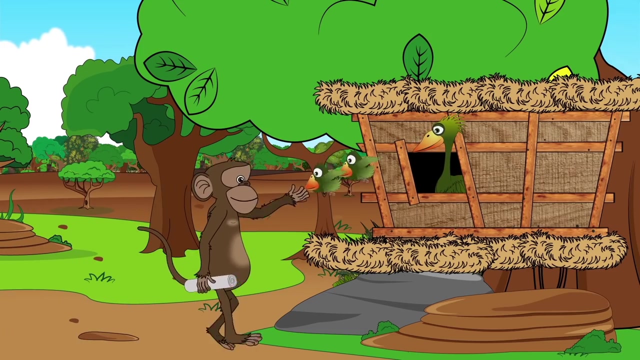 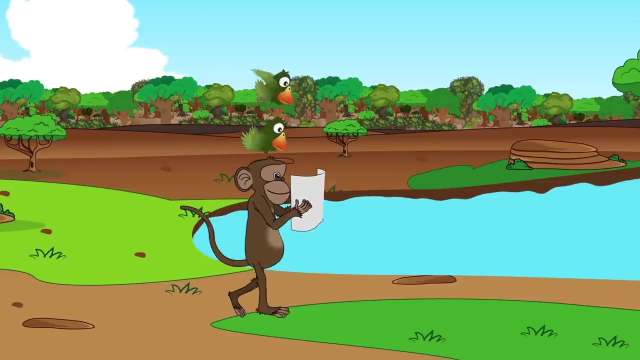 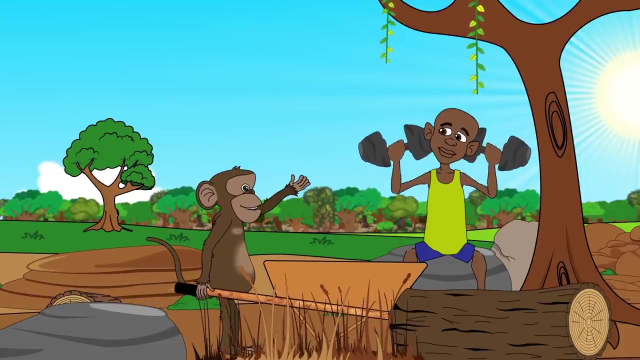 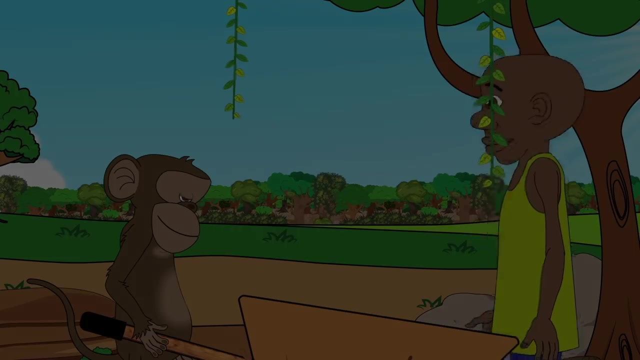 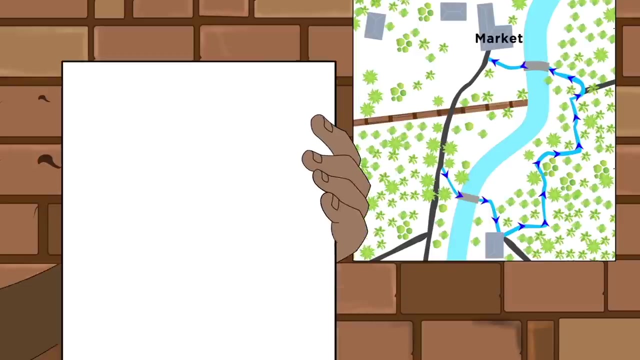 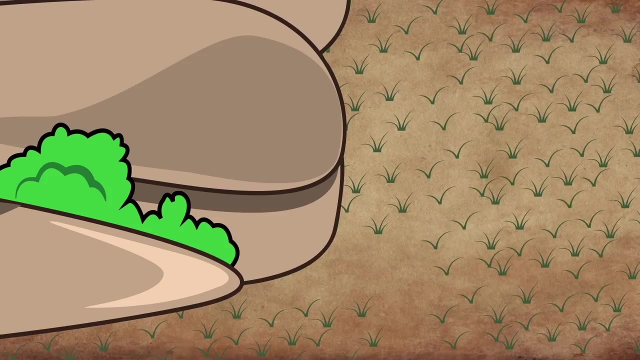 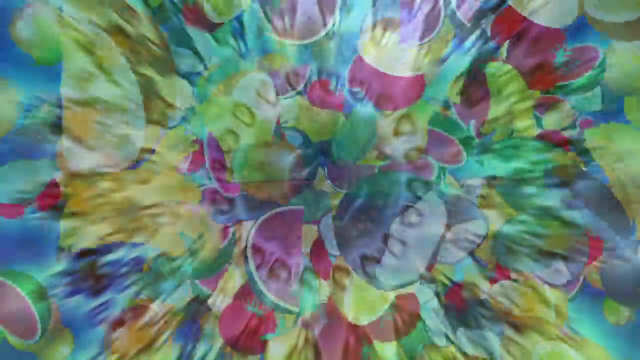 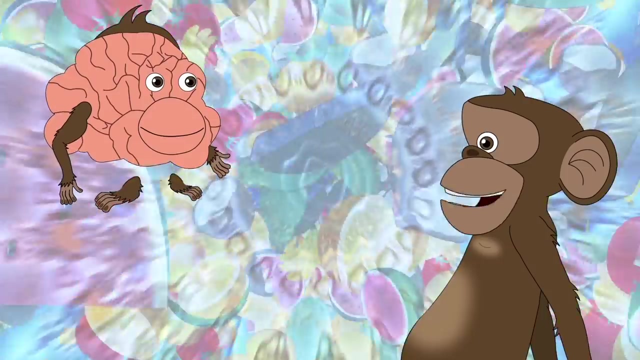 Thank you. Thank you, I think I'm ready. I'm going to go for the big map. Woohoo, You can do it. Ngerere, Watch out Huh. Hey, Ngerere, check this out. 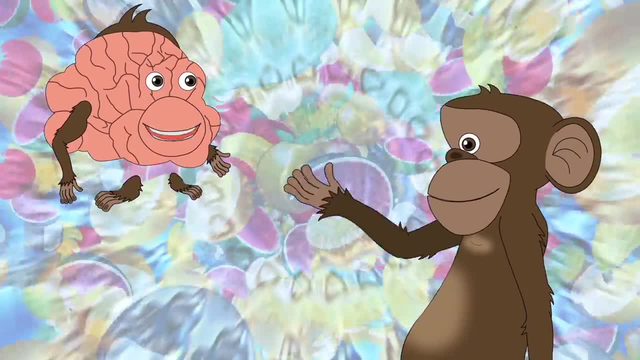 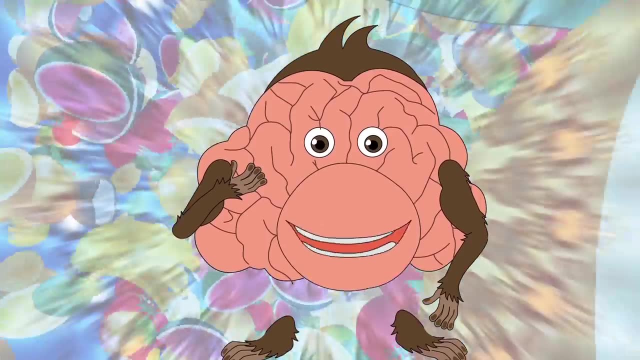 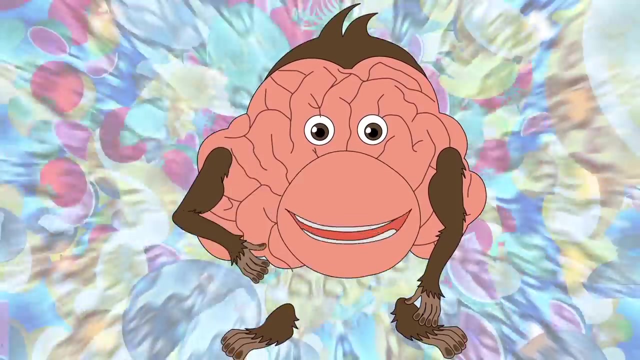 Wow, Brain, you're looking awesome. Thanks for the exercise, but I didn't really exercise you. I just read lots of maps. That is exercise for me: Doing hard things that you can't quite do well yet You've been doing lots of that and I've been getting super strong. 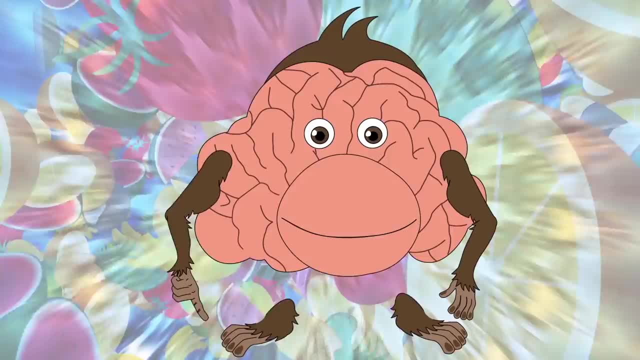 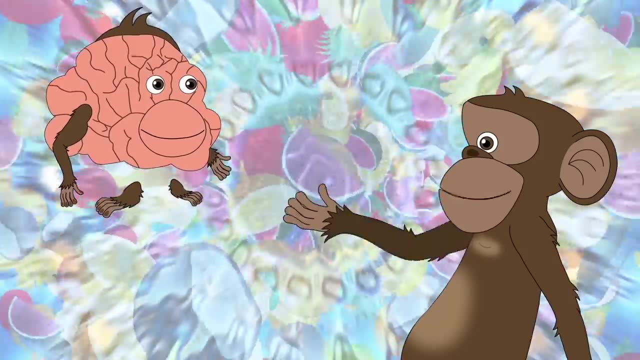 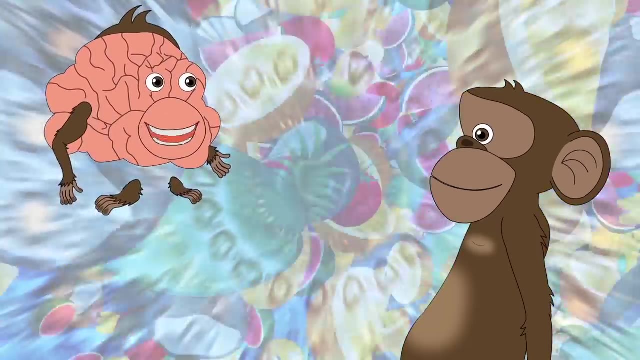 You see, when you learn something new, you create a pathway in your brain. That's me, And a pathway is called a neural pathway, Kind of like when I make a new path in the forest. That's right, And then the more times you practice doing the thing, 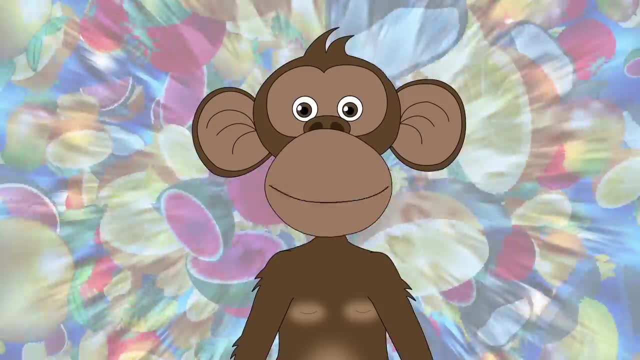 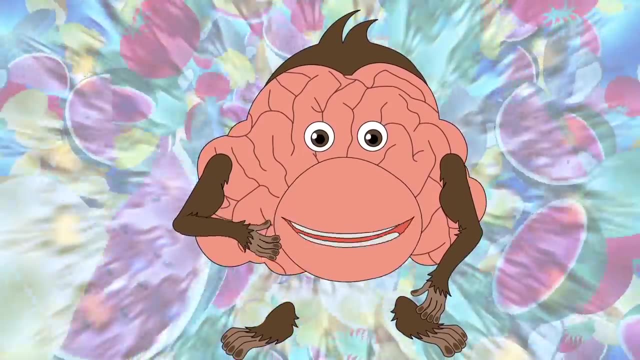 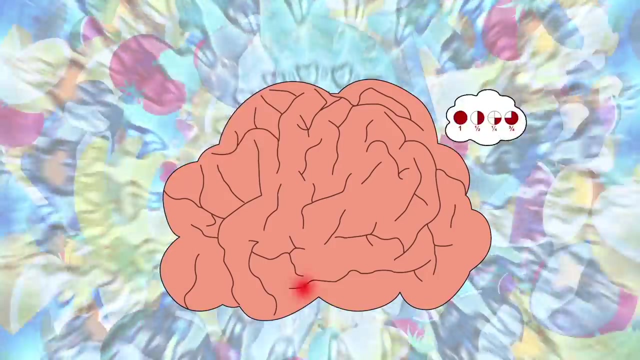 the easier it becomes to travel that neural pathway, Just like the more times I run along a path, the easier it becomes to travel. Exactly, You've got lots of paths already, Like roots, fractions, decimals and now maps. 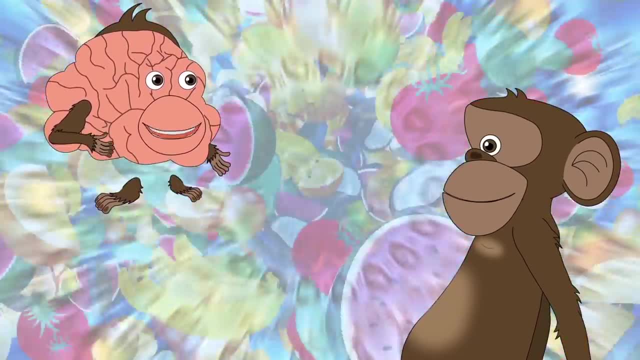 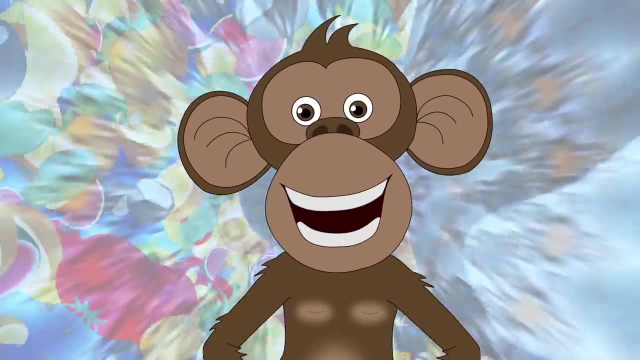 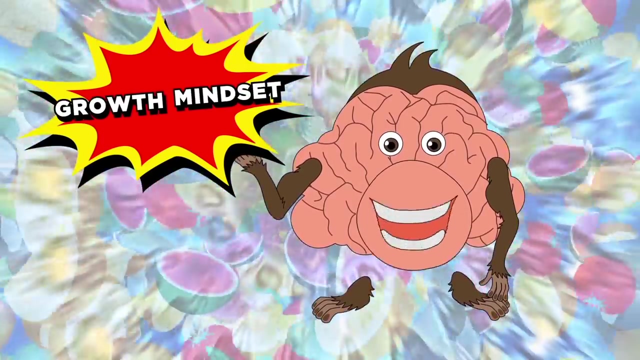 That path is really clear now because you've been using it a lot lately And now that you know how you can grow your brain, you can keep doing it to learn anything. Wow, It's called having a growth mindset, Believing that you can grow your smarts, your skills and your talents. 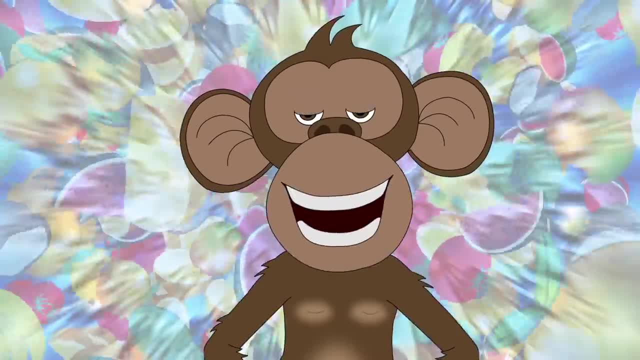 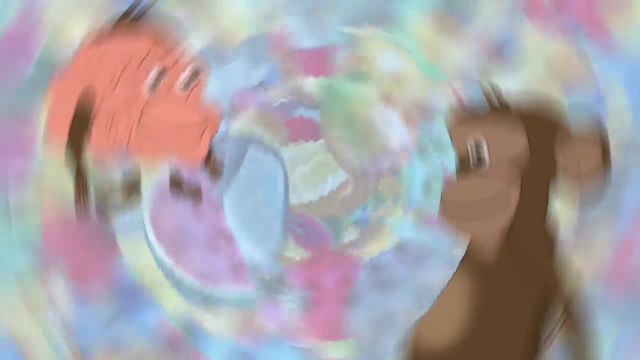 And all it takes is hard work and practice. Wow, I love it. Growth mindset- G-dare it. G-dare it, Hey, G-dare it. Are you okay? Are you okay? Hey, G-dare it. 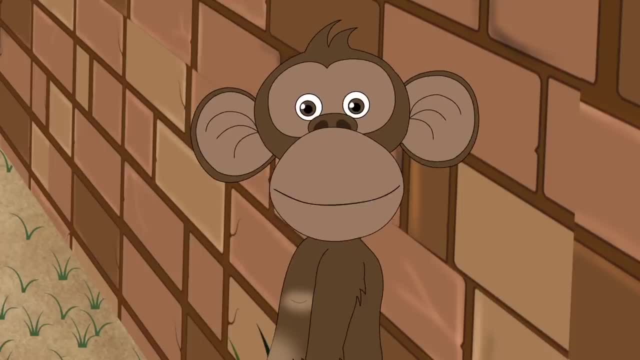 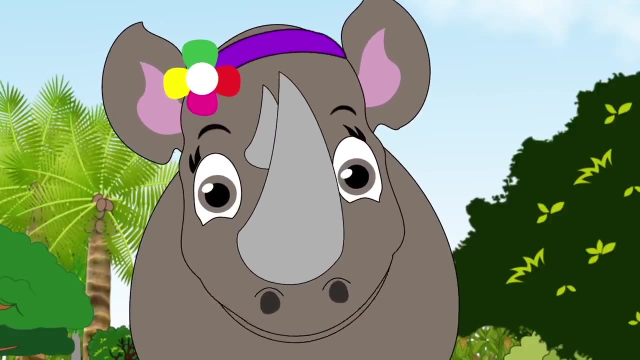 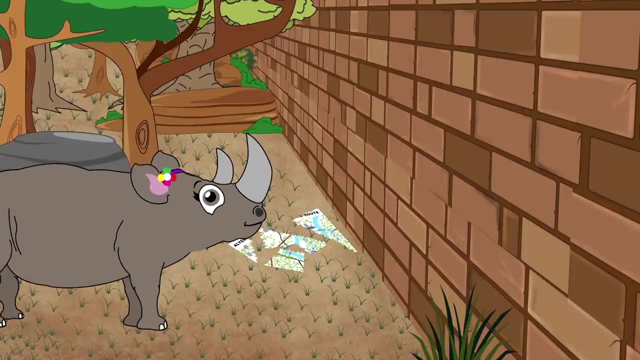 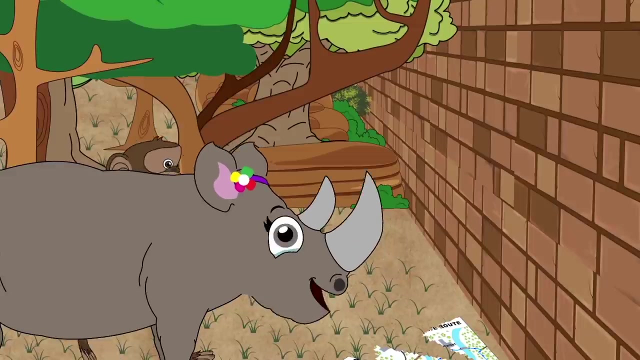 Phew, You're out cold. Yo Fafa, Come on. How many times have you bashed your head against this wall? 157!, And does it look any closer to falling down? Hmmno, But my daddy says I'm the best young basher. 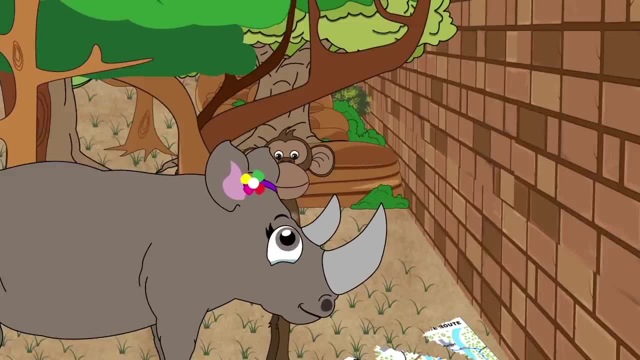 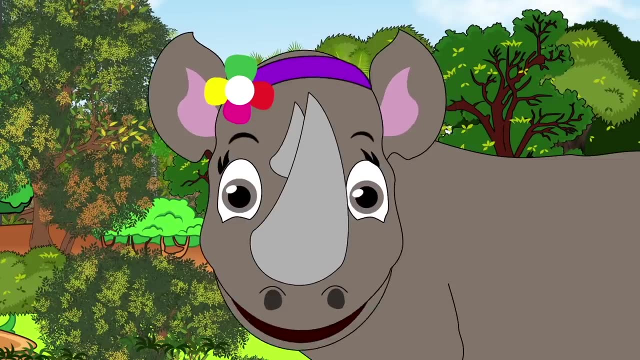 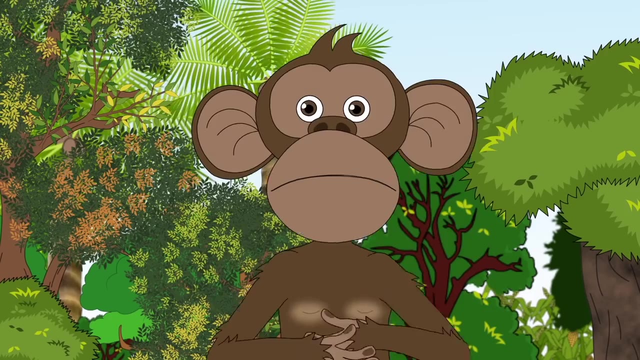 in the whole forest. Yes, I know, But some walls aren't meant to be bashed down. Sometimes you have to find another way around them. But how Well. luckily there's a map to help us. No, 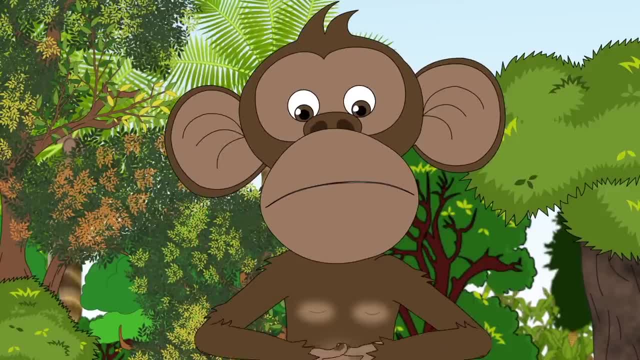 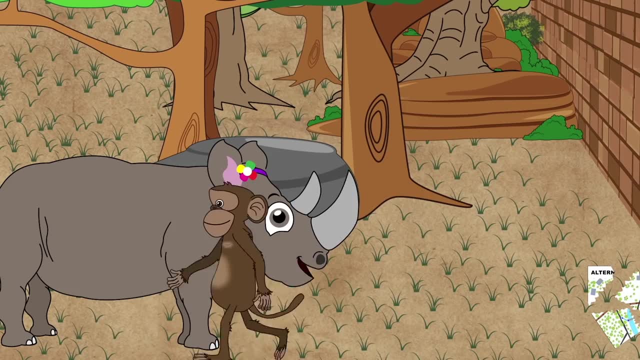 No, no, no, no, no. My map, My map. No Wait, This is an opportunity To get lost in the forest and never find our way out again. No, Fafa, It's an opportunity to try something new. 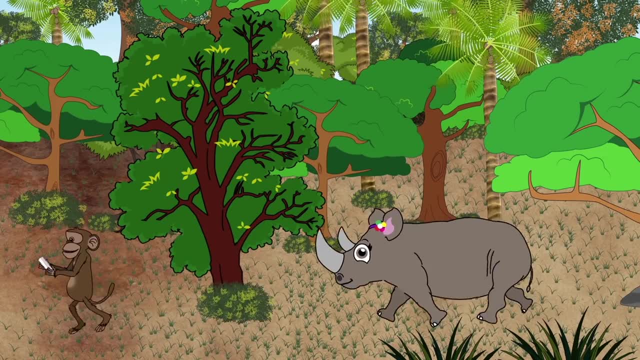 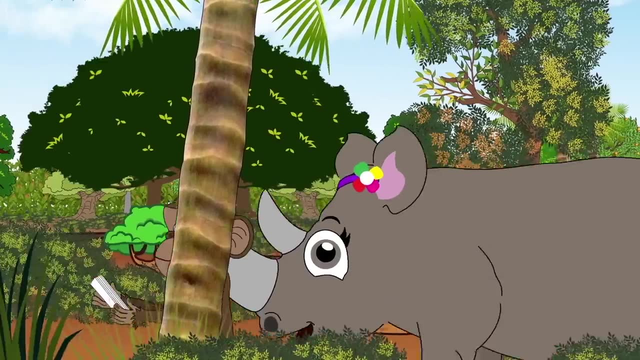 Come on, Fafa, We're going to make our own path And I need a basher to help me out. Oh Me, Oh, I can bash. My daddy says I'm the best young basher in the whole forest. 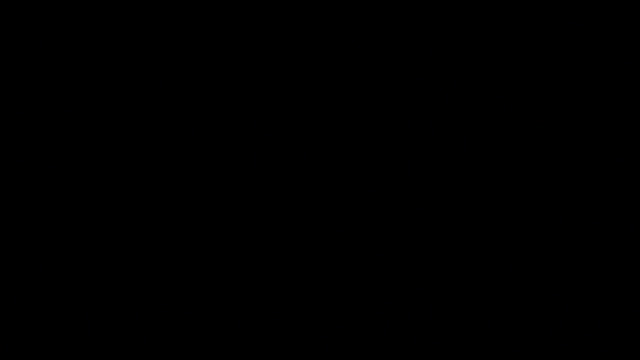 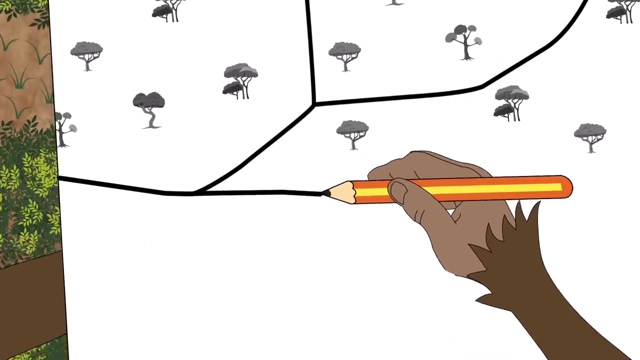 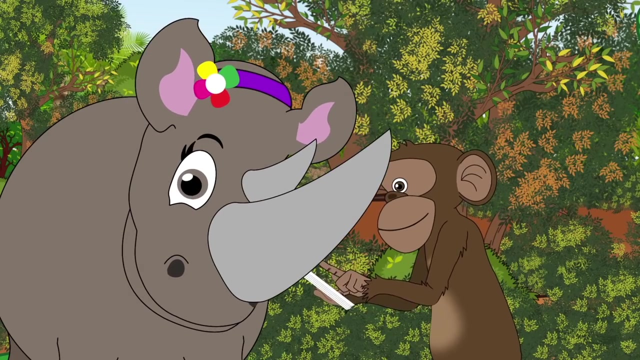 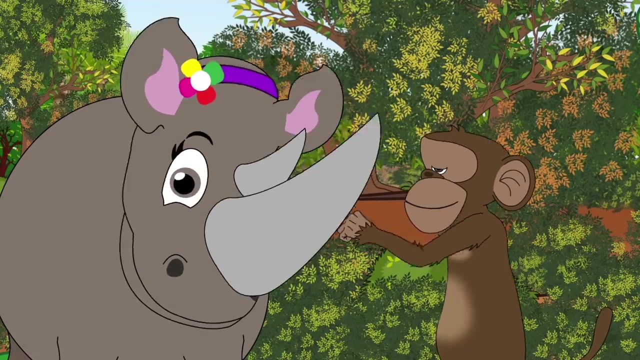 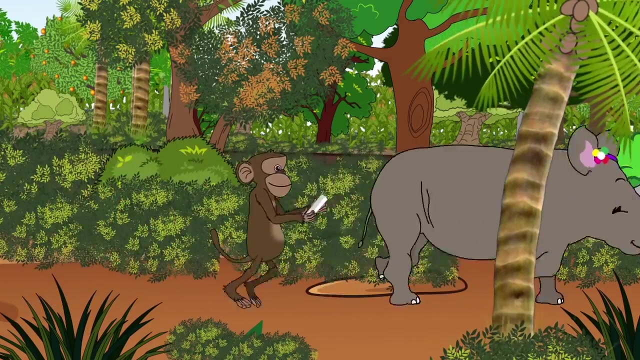 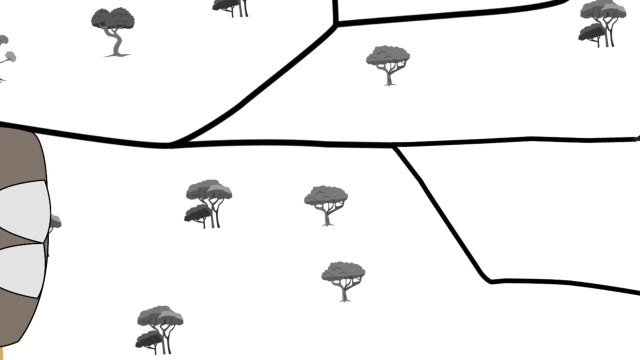 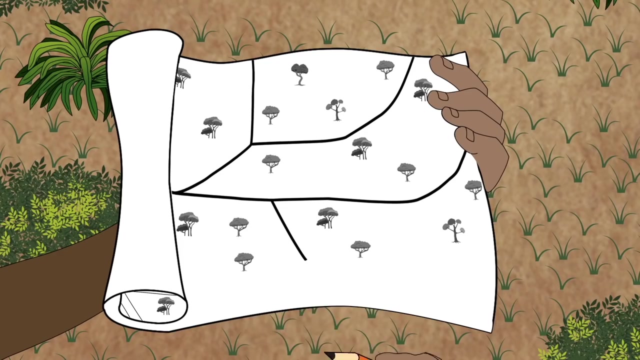 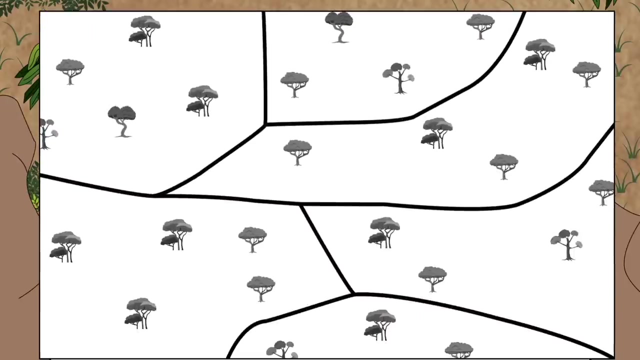 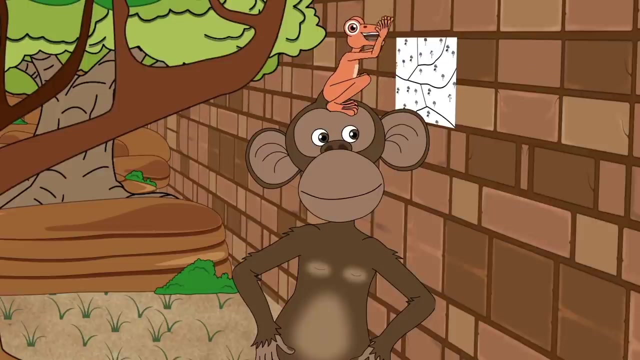 In the whole forest, The whole forest. I get it. That shows our path. Yes, goin' our own way. Ah ت heirتي irim. Thank you, And Aaron, that's a great map. You must have worked really hard to make it. 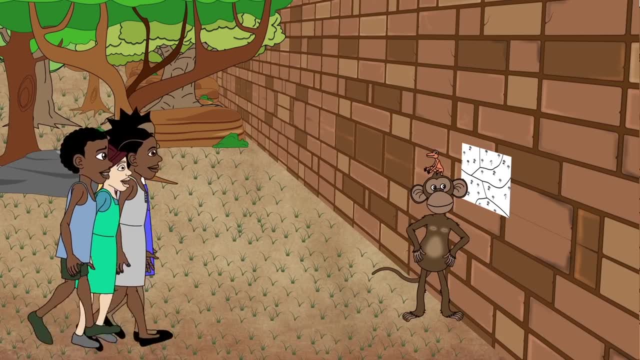 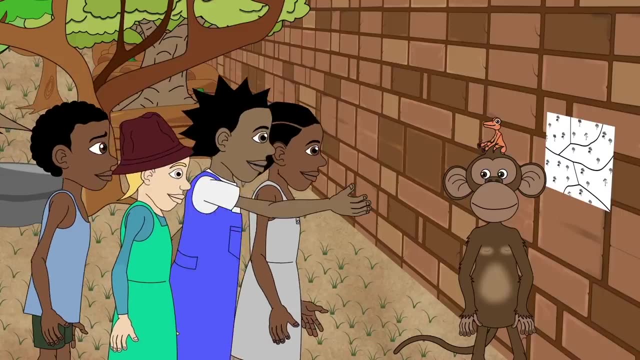 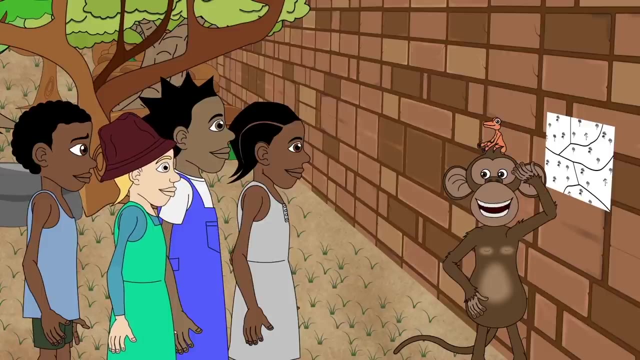 Wow, Wow. It's a map. Who made that map? Fafa, and I did it. I didn't know you were a map maker. Well, I had to grow my brain just a little bit to do it. I thought it was impossible, but then my brain talked some sense into me. 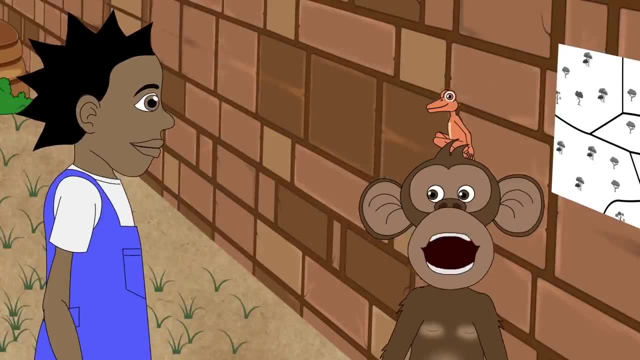 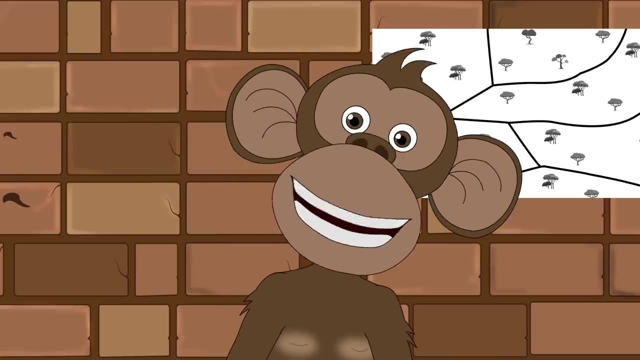 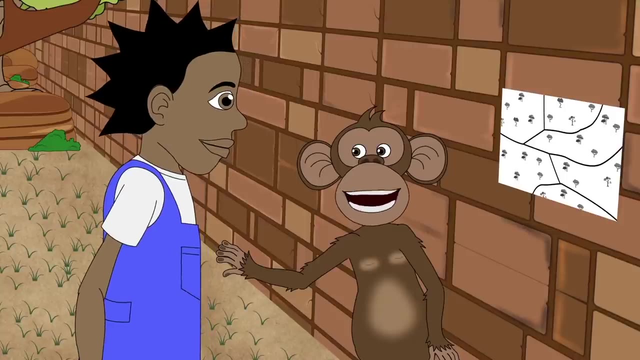 Huh, No, Kiduchu, When you grow your brain, it doesn't get bigger in size. okay, It builds more pathways and makes more connections so that it can do more things, Just like how Fafa and I created new pathways in the forest to connect more places. 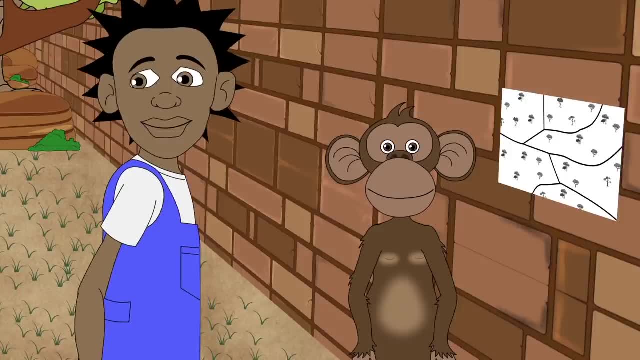 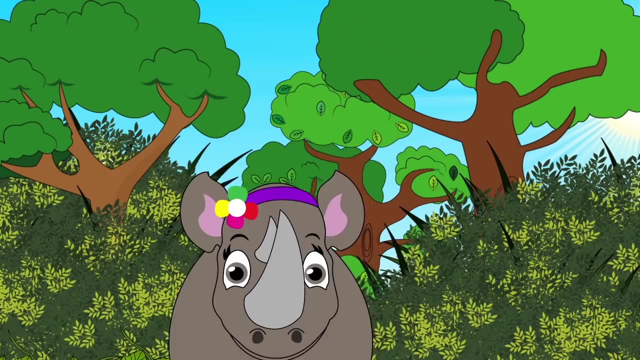 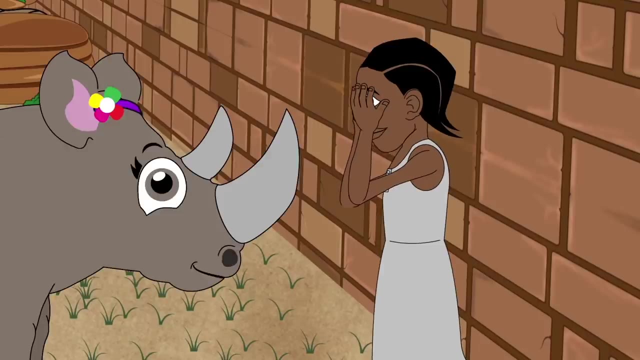 Who's Fafa? Fafa Coming. Hi, I'm Fafa and I'm learning to stop before I bash into things. Well, uh, good job, And thanks for stopping before you bashed into me. Thank God, Aaron. 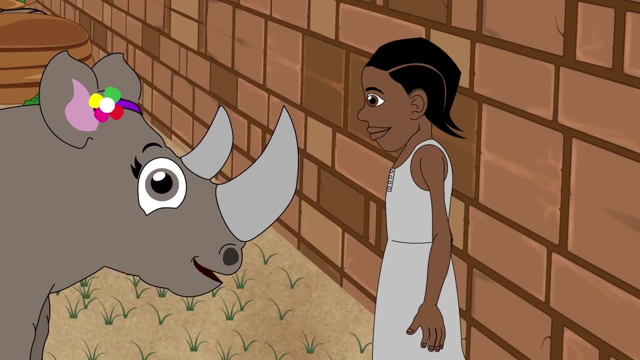 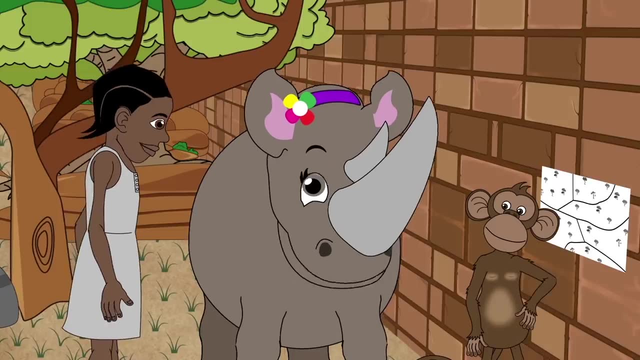 He's the one who helped me see that I don't have to be good at just one thing. I can be a great basher, but I can learn how to stop too. It's all about. It's all about having a growth mindset. 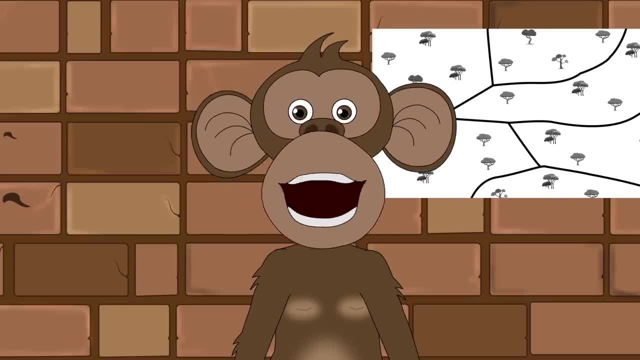 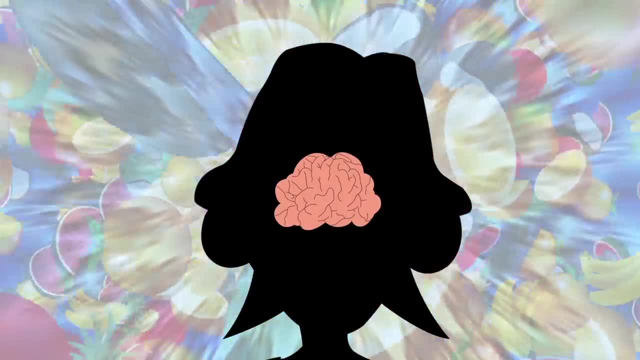 Close your eyes and think about something you really, really, really want to learn. I want to learn to read music. It's like a language I don't know. These music notes are so confusing To read them. my brain's gotta grow. 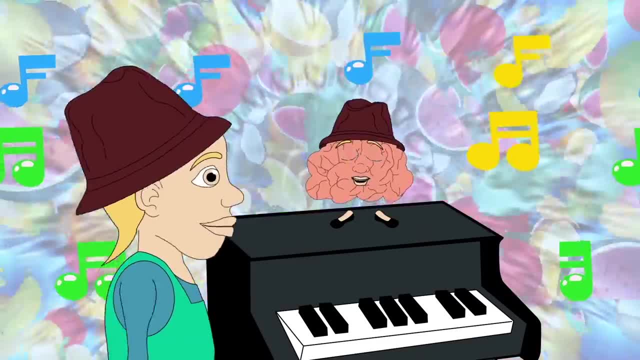 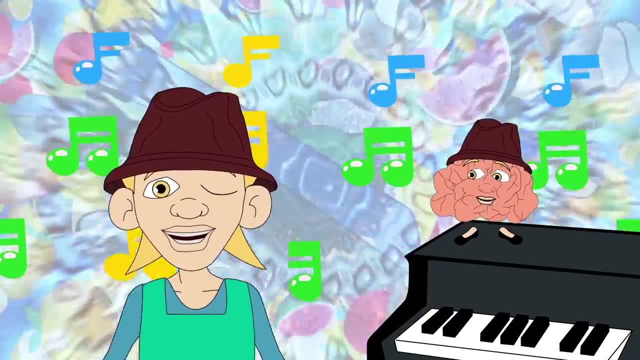 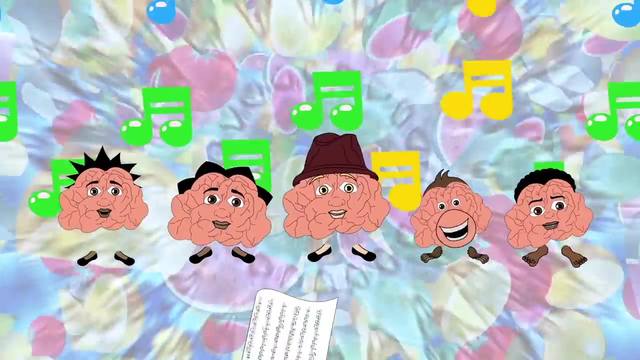 Reading music is a difficult thing- All those notes and lines- But anyone can learn to do it. You just gotta try. Maybe it will be hard work, It can even be fun. Take it step by step, One by one. Grow your brain. grow your brain. 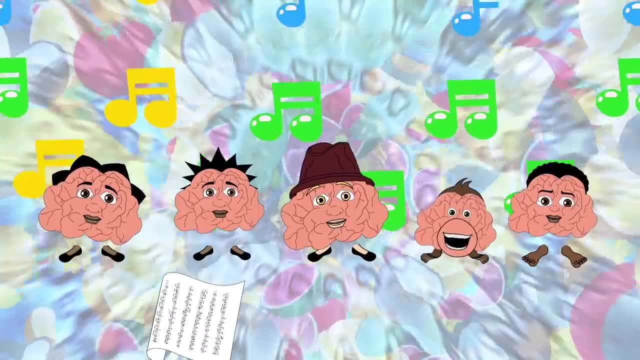 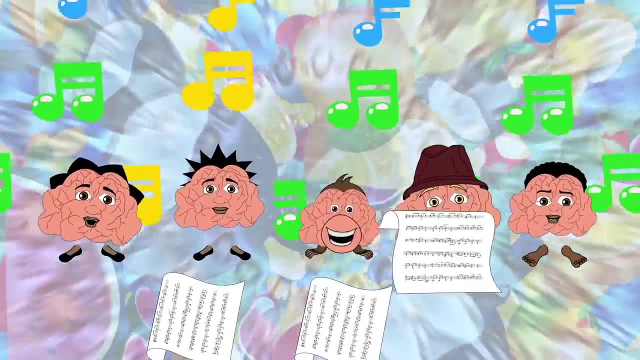 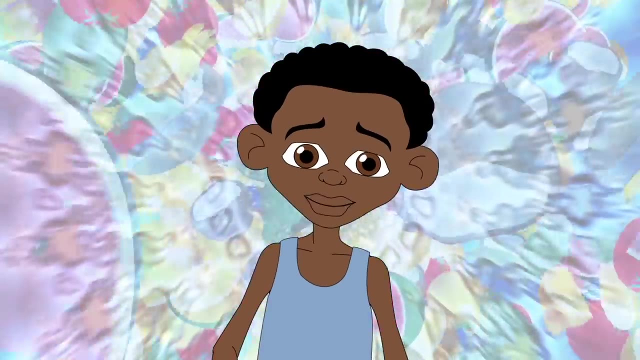 Give it work to do. Grow your brain. grow your brain, Learn something new. Grow your brain, grow your brain To be a smarter. you Give a challenge a go And hope your brain glows. I used to be the best at maths. 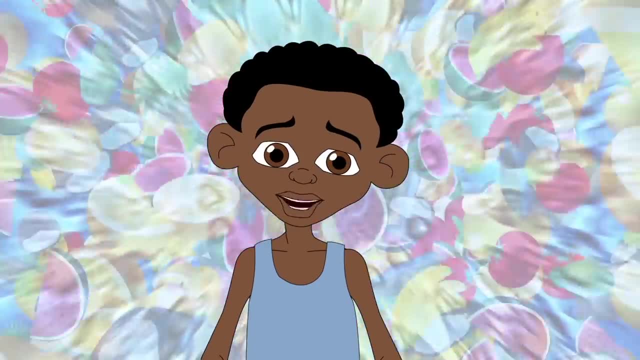 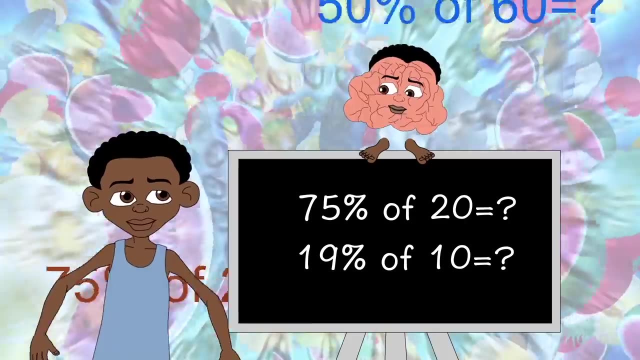 Fractions, decimals- they were easy, But then, per se, I learned a lot. But then percentages came along, And now maths is no longer for me. If you stick to what you know and what comes easily, I'll never get a chance to grow, and that's not fair to me. 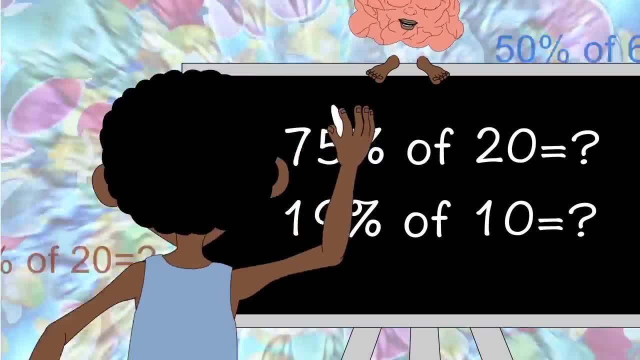 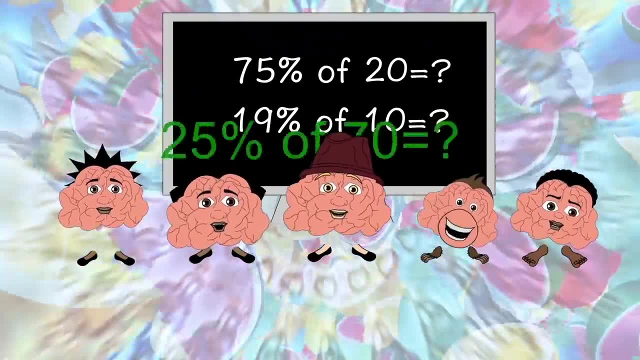 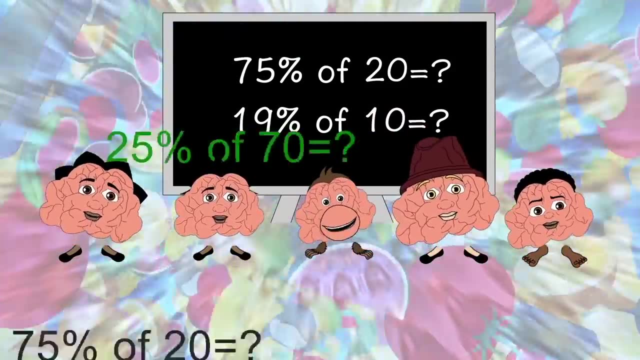 When you try out something new, it challenges me too. That's what I need to help me grow and grow. Grow your brain, grow your brain. Give it work to do. Grow your brain, grow your brain, Learn something new. Grow your brain, grow your brain. 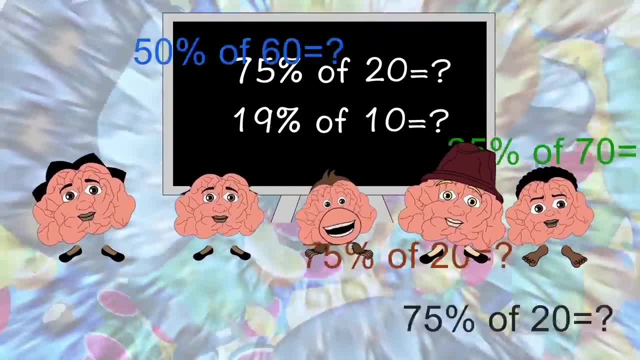 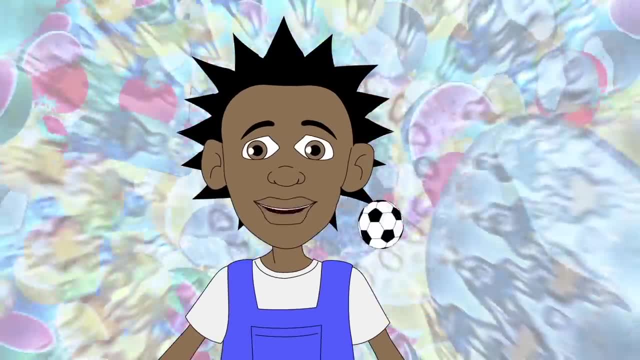 To be a smarter. you Give a challenge a go And hope your brain glows. Well, you all know I'm a football star. I score lots of goals all the time, But only using my super left foot. I'm useless with the right. 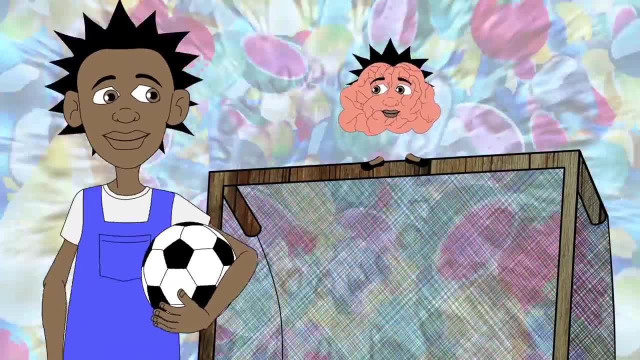 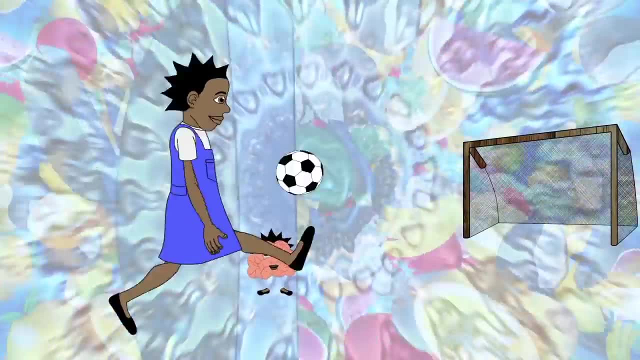 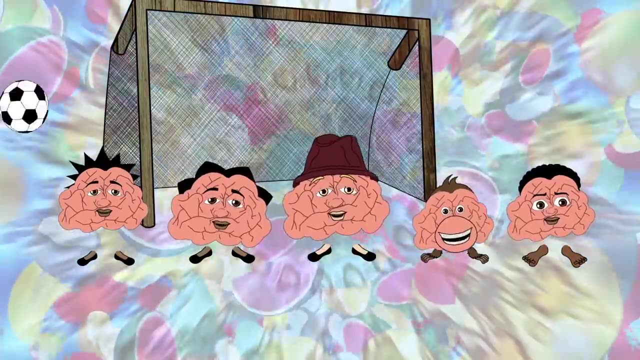 The only way to build new skills is to practice. It's not always easy, but you can do it. Don't be afraid to fail. You get there in the end. All you have to do is grow your brain, my friend. Grow your brain, grow your brain. 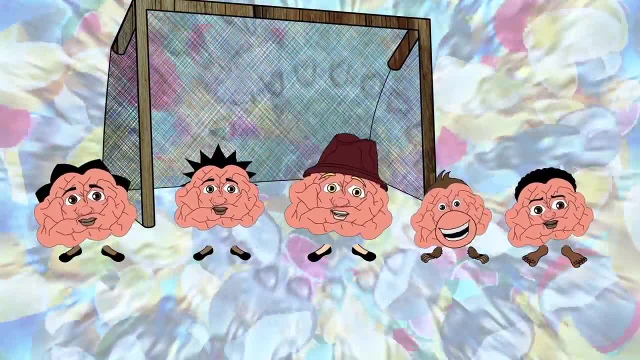 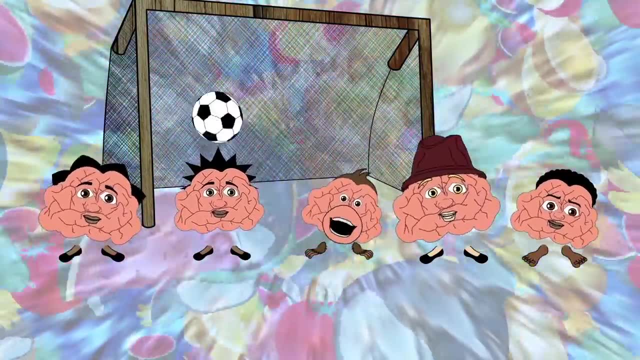 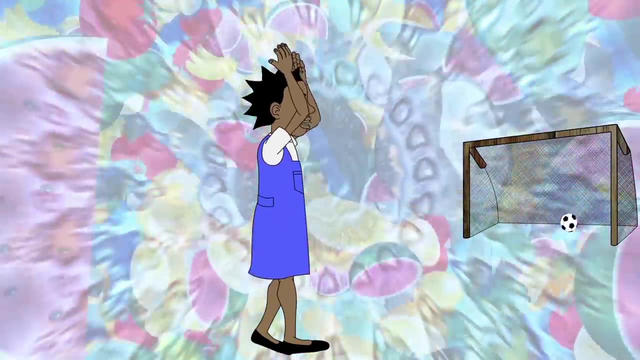 Give it work to do. Grow your brain. grow your brain, Learn something new. Grow your brain, grow your brain To be a smarter. you Give a challenge a go And hope your brain glows. Believe in yourself, even if you can't do it yet. 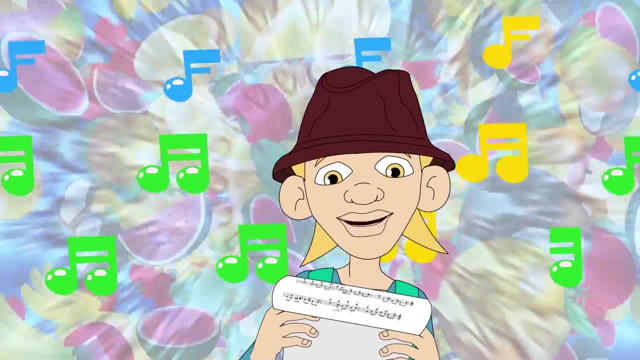 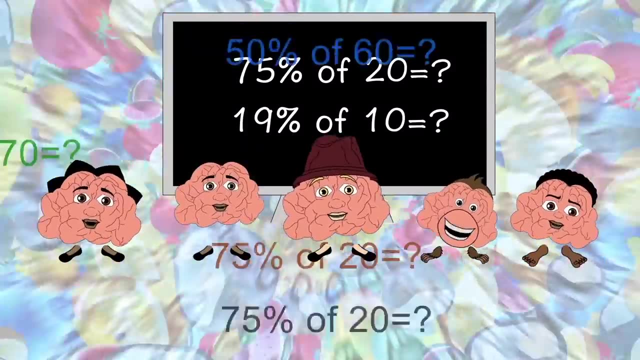 Believe that you can learn how It's called growth mindset. Grow your brain, grow your brain, Give it work to do. Grow your brain, grow your brain, Learn something new. Grow your brain, grow your brain To be a smarter you. 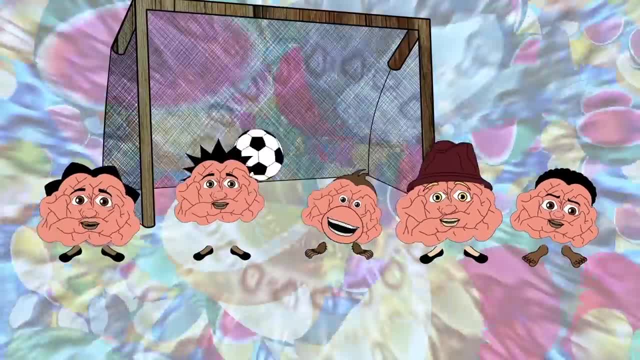 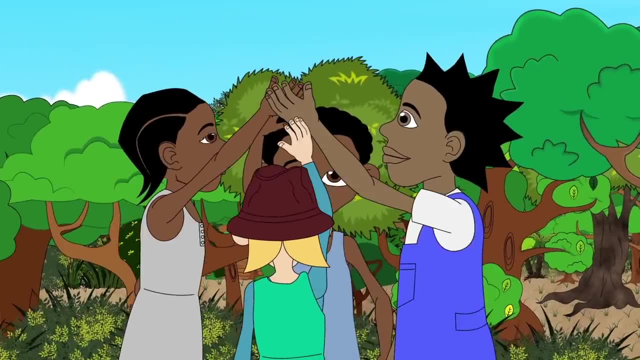 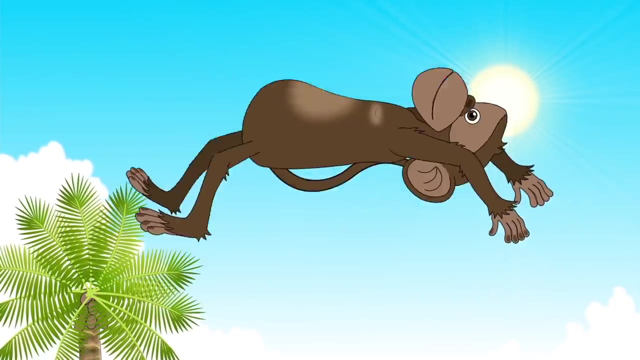 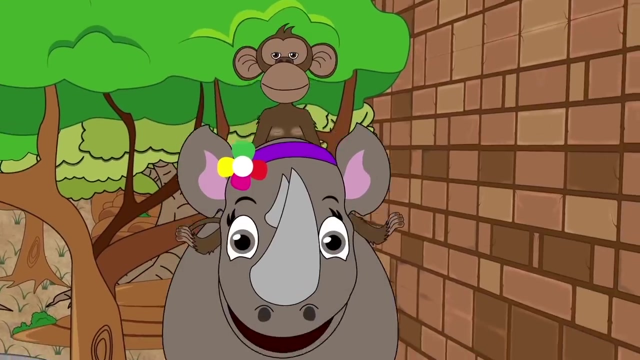 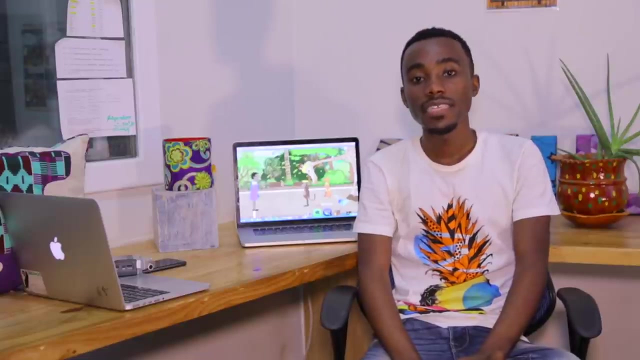 Give a challenge a go And hope your brain glows. Whoa To growth mindset. Nice, stop Fafa. Yeah, Hi, my name is Mohamed. I am an animator As far back as I can remember. I always wanted to create cartoons. 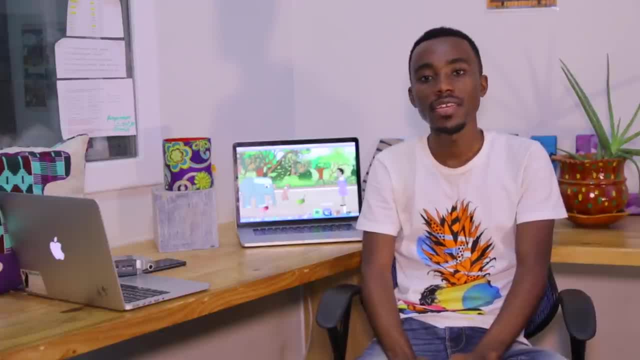 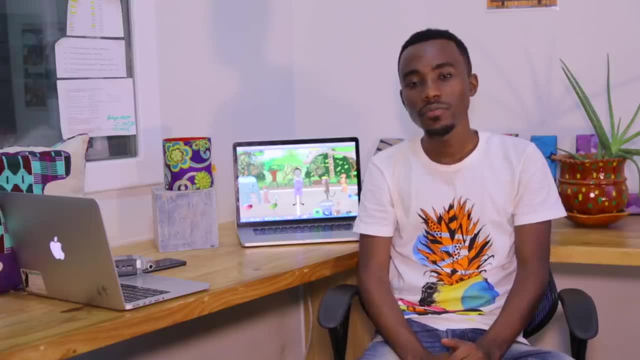 Since, when I was around 12 to 13,, I started getting into drawing And by that time I thought to be an animator. I had to have talent or be good in drawing, So I joined a film school And started taking animation lessons. 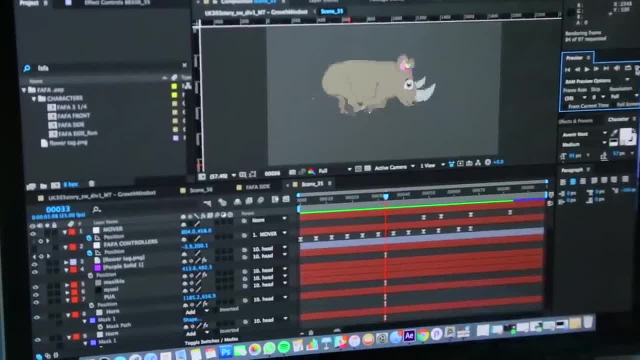 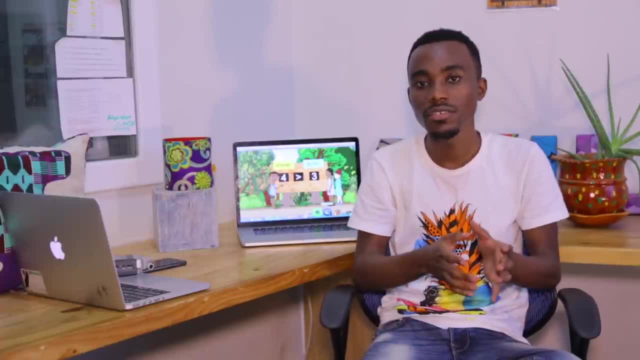 But I was having issues with understanding some softwares Which were hard for me to understand. Still, I never gave up. I tried hard and found some other ways to learn those softwares and to master them So I can be good in it and still grow my mind, so I can reach my dreams. 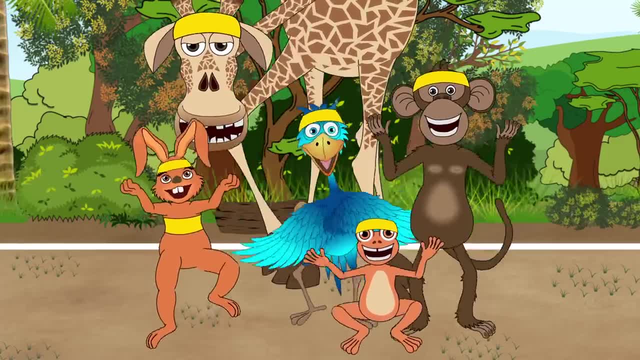 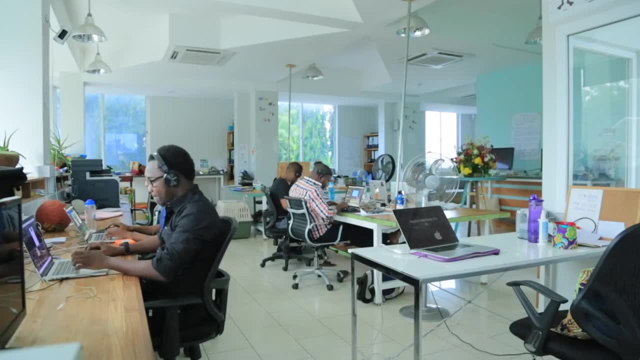 And here I am creating cartoons for all the kids And I hope you enjoy it. So you see, you have to grow your mind by trying different ways to get solutions So you can reach your dreams If you stick to what you know. 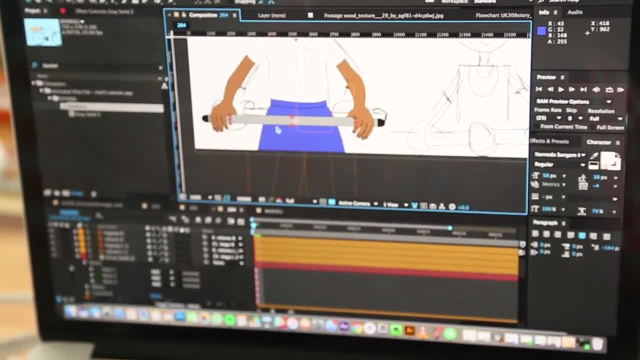 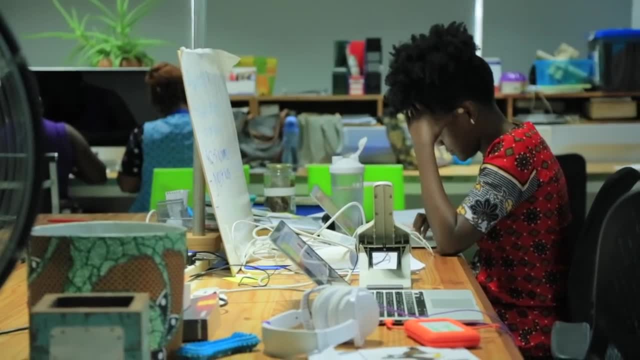 And what comes easily, I'll never get a chance to grow, And that's not fair to me. When you try out something new, It challenges me too. That's what I need to help me grow and grow. Grow your brain, grow your brain. 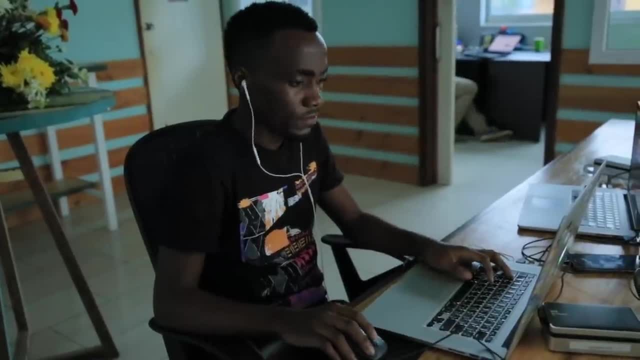 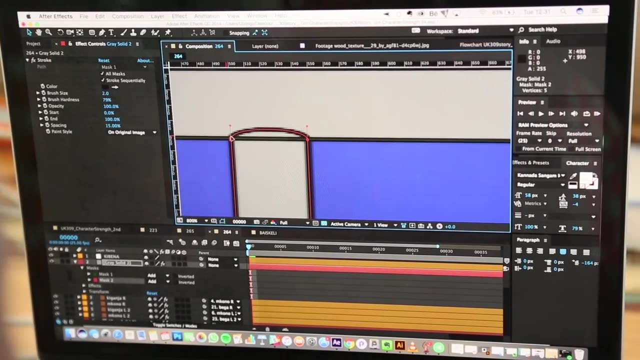 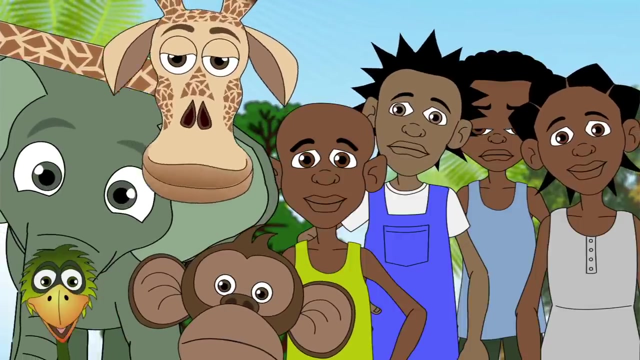 Give it work to do. Grow your brain. grow your brain, Learn something new. Grow your brain, grow your brain To be a smarter. you Give the challenge a go And help your brain grow. Believe in yourself, Even if you can't do it yet. 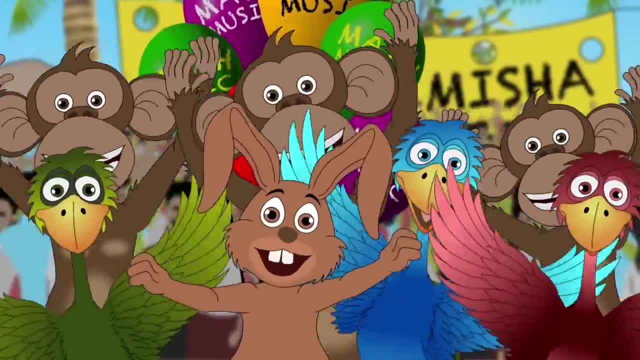 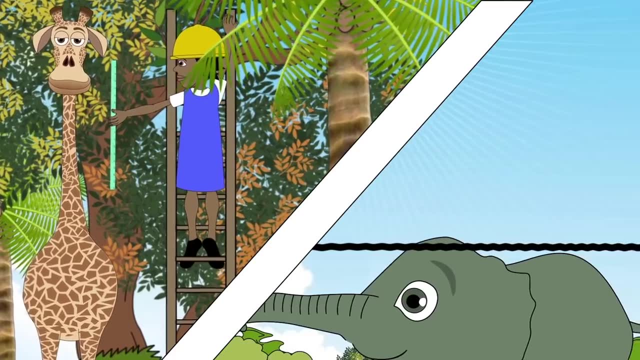 Believe that you can learn how It's called growth mindset. Grow your brain, grow your brain, Give it work to do. Grow your brain, grow your brain, Learn something new. Grow your brain, grow your brain To be a smarter you. 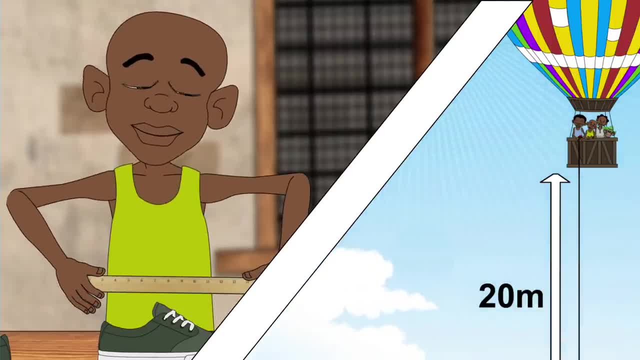 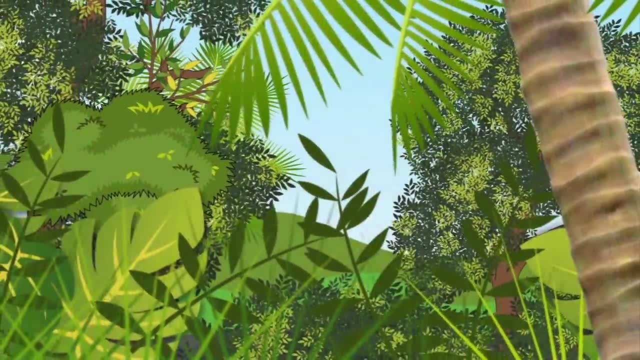 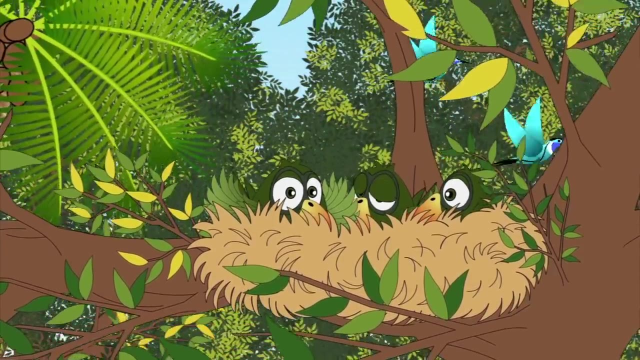 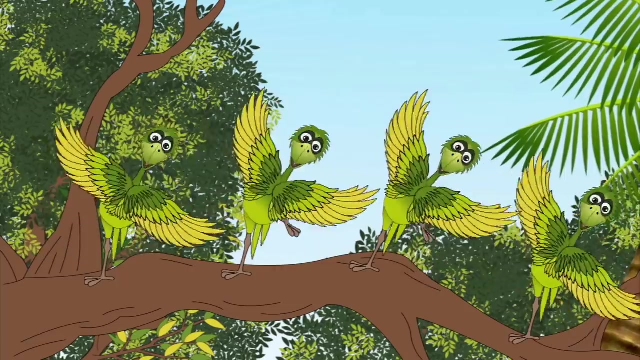 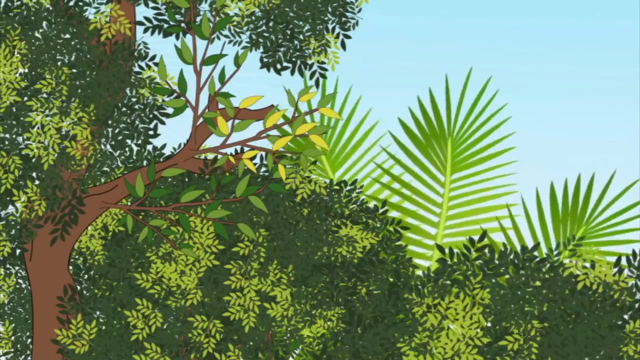 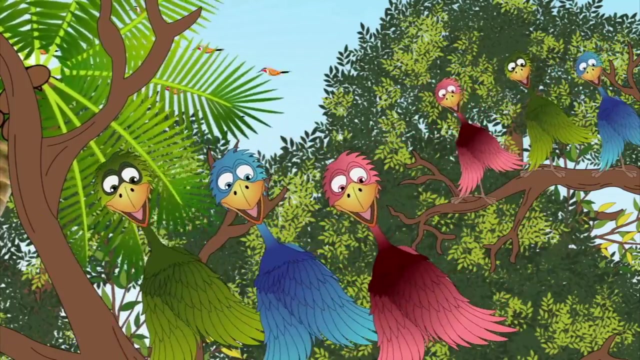 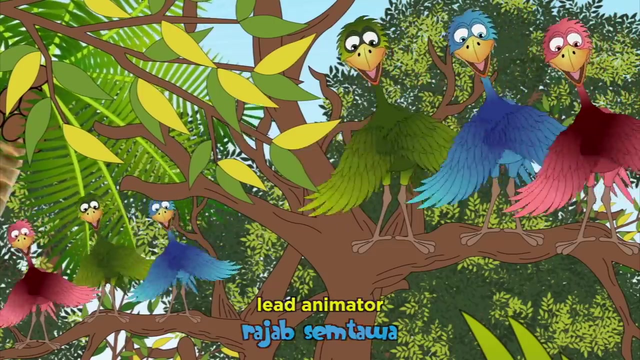 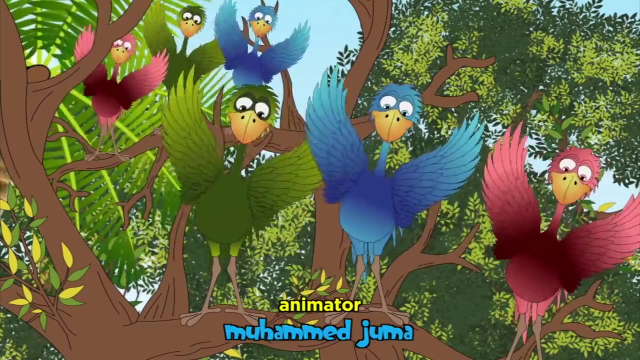 Give the challenge a go And help your brain grow lives. 3. je j k dy da e ny die اب mother. okay I. Mathematics, how I love it. Mathematics, hey, yeah. Sing about the magic of mathematics. Mathematics, hey, yeah. 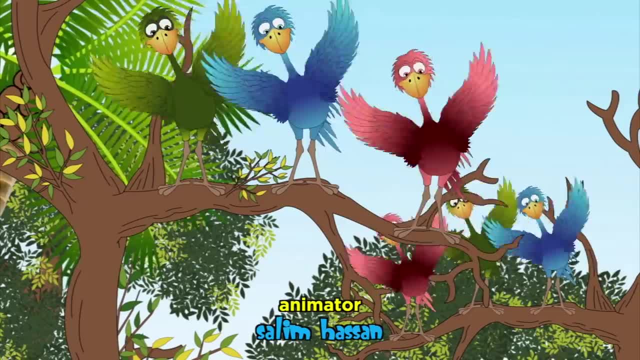 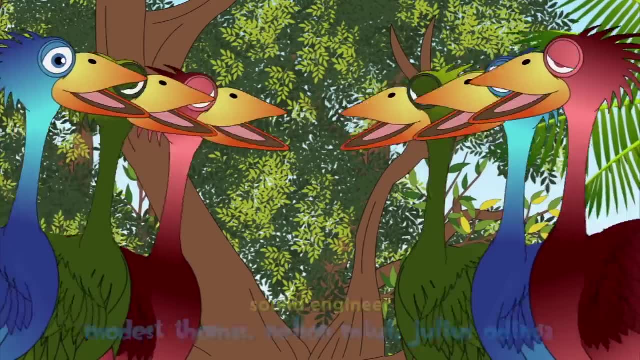 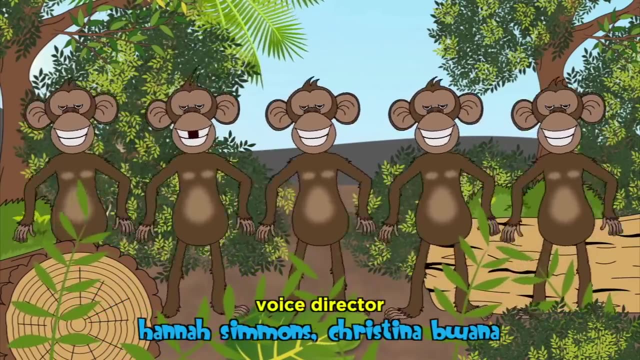 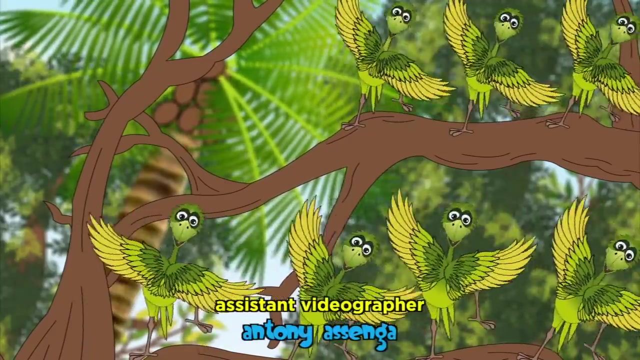 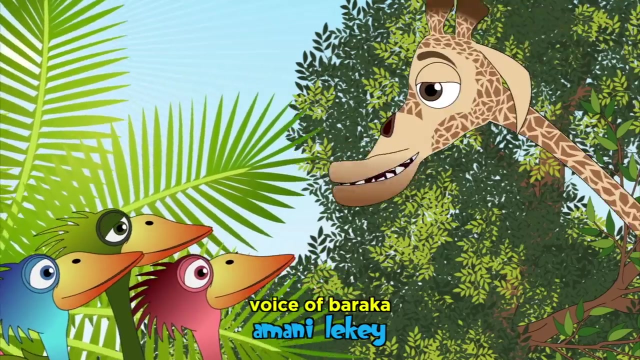 Making number magic with mathematics. Mathematics, hey, yeah, Sing about the magic of mathematics, Mathematics, hey, yeah. What is mathematics? Mental acrobatics Every day, all the time. just use your mind. You use math when you measure width and length, solving problems using mental strength. 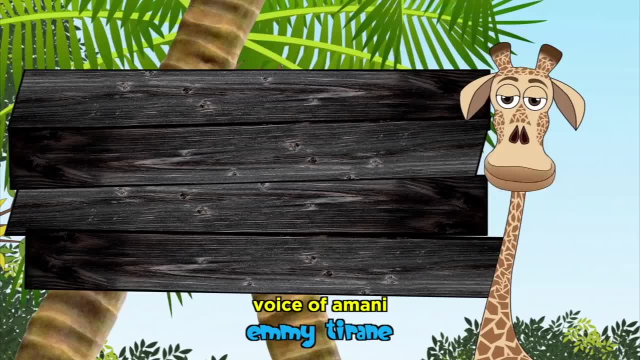 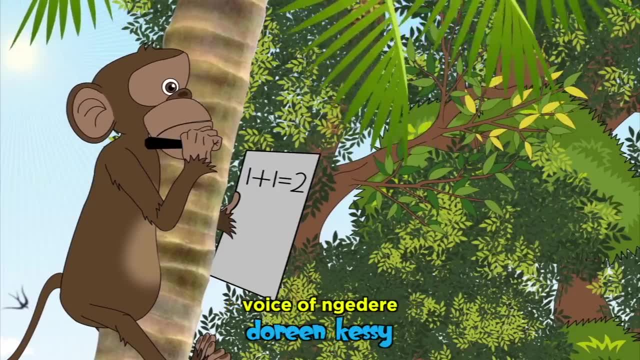 Use number operations like multiplication. The number you'll find is like magic from your mind. Math is a part of everyday life. Just add, subtract, divide and multiply. Can you subtract? What's the problem? Did you get the answer? Just use your brain and you can do it, sir. 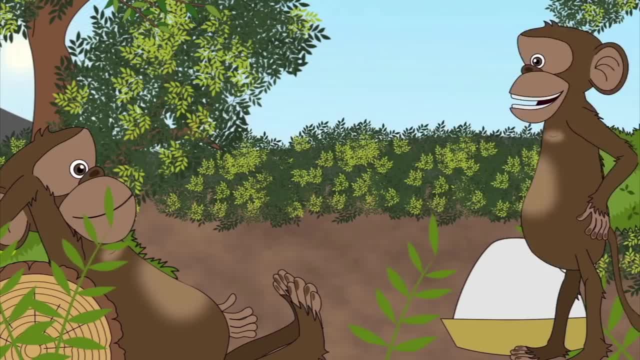 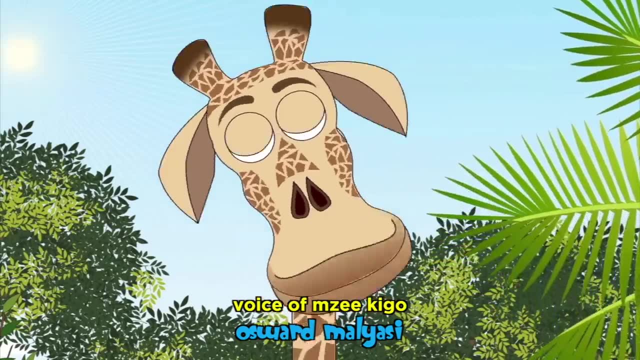 Now, don't you rush it, Just take it slow. You must be careful, Don't you know? You use math for all things in life. When you eat ugali, you count your bites. In a parade, count the steps you take. Just listen. when I rap, I'm using math. 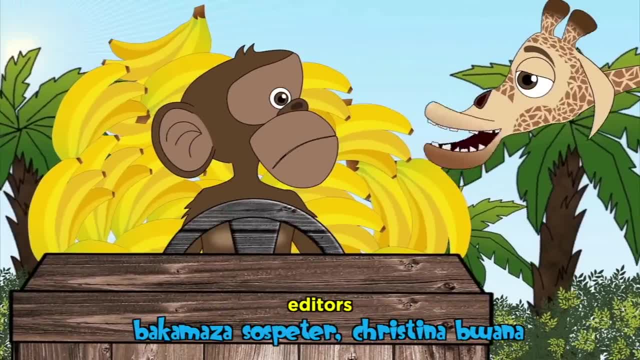 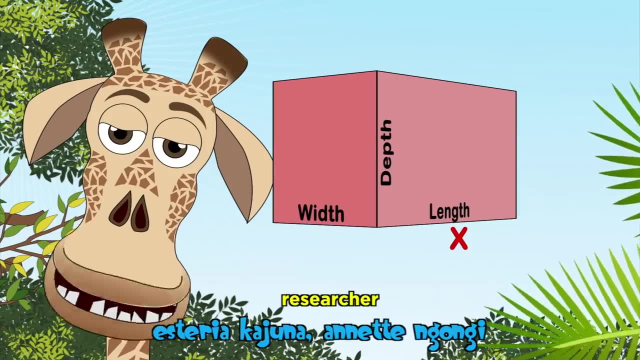 Calculate the distance when you drive your car, so you will know if you've gone far. Here's something else for you to count. Can you count the teeth in my mouth? We can measure width, length and depth and represent with X, Y and Z.